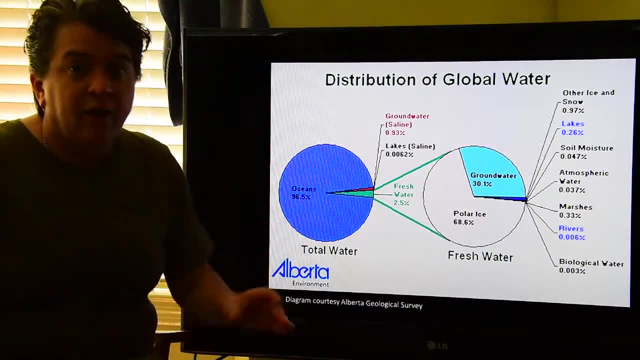 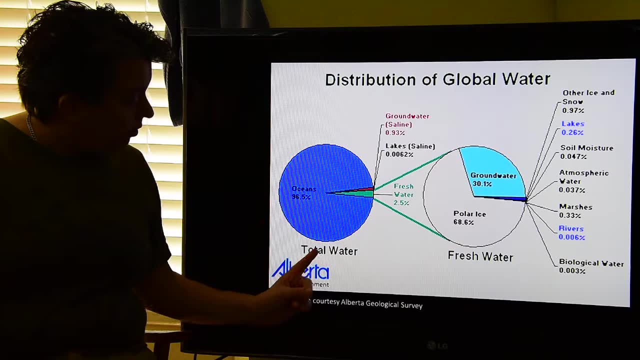 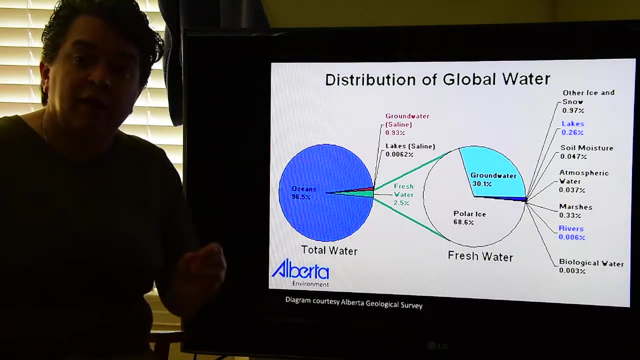 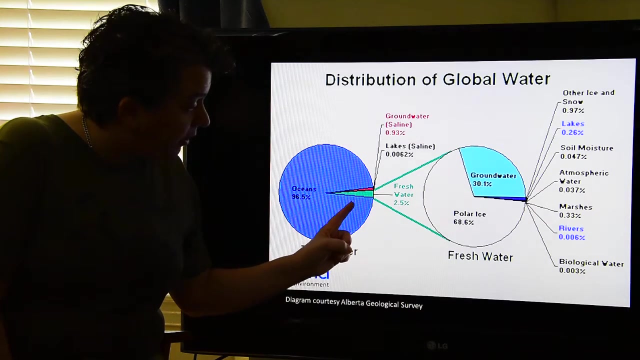 If you read a book and the numbers are slightly different, it's because they're estimates. Basically, the big picture is: let's look at this: This is total water on Earth. Most of it is in the world's oceans. Most of it is actually salty. Fresh water on our planet is this tiny little area right here. 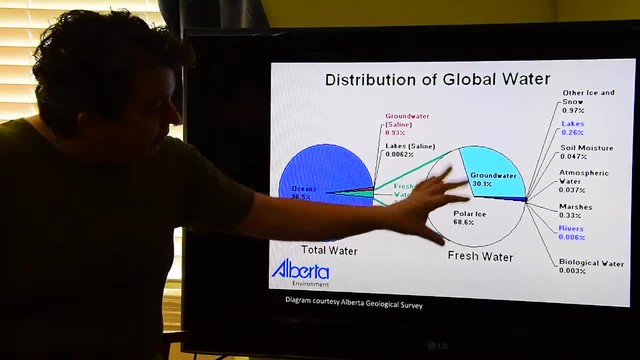 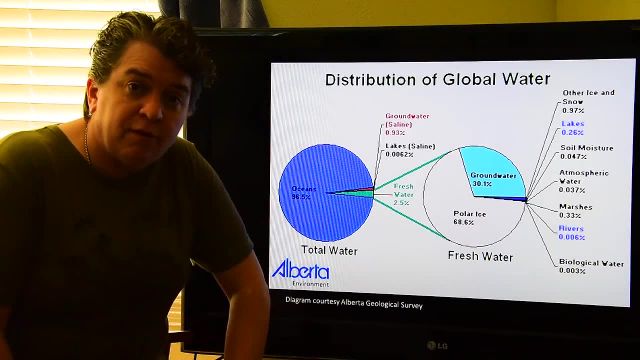 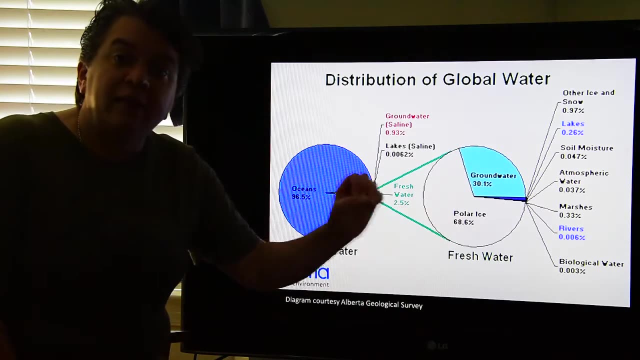 Let's look at that fresh water. If we just look at fresh water on Earth, most of it is stuck in ice. Most of it is basically the ice that's covering Antarctica and Greenland and places like that. Of the liquid fresh water, most of it is underground. 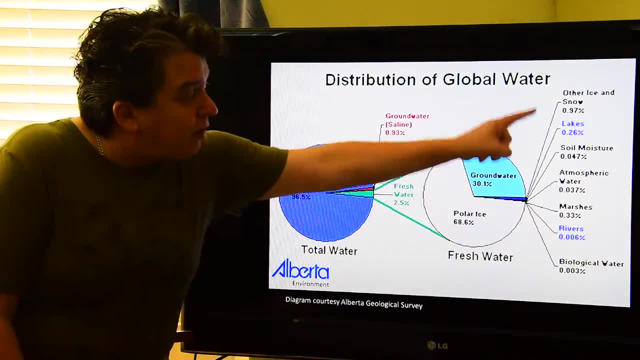 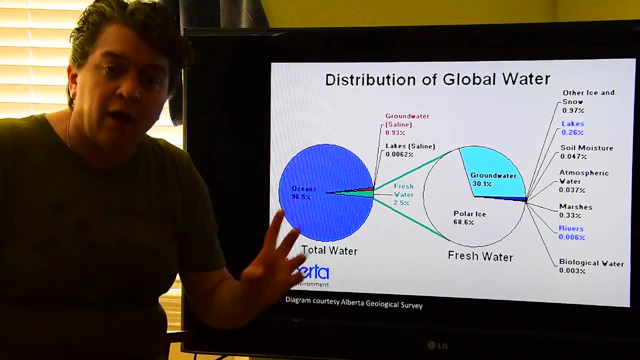 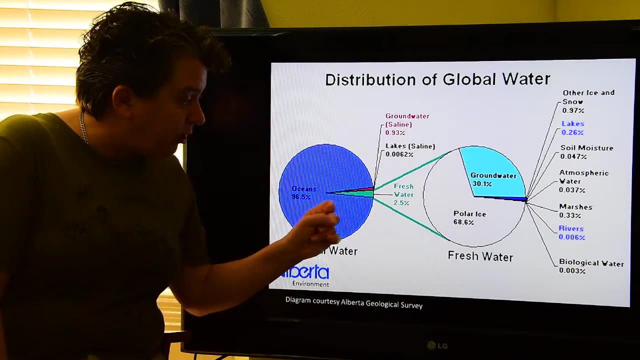 Just this tiny little amount is the amount that is in the atmosphere or in lakes and streams and swamps and things like that. You guys don't need to remember these numbers, But you should know. most water on Earth is salty. A small amount is fresh. 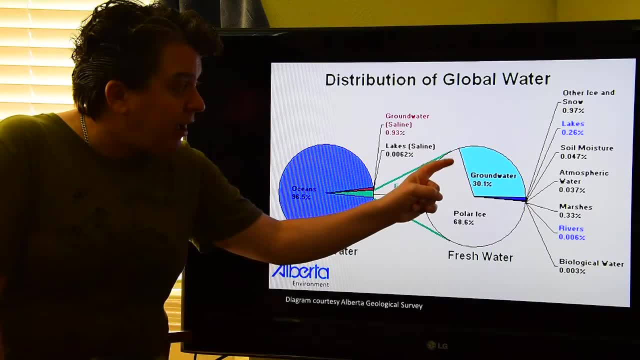 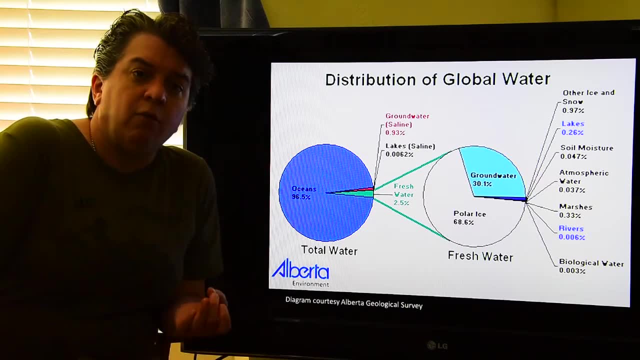 Of the fresh water, most of it is frozen And the liquid part most of it is underground. Now, just because water is frozen today, or it's in the oceans today, or it's underground today, doesn't mean it's going to be there forever. 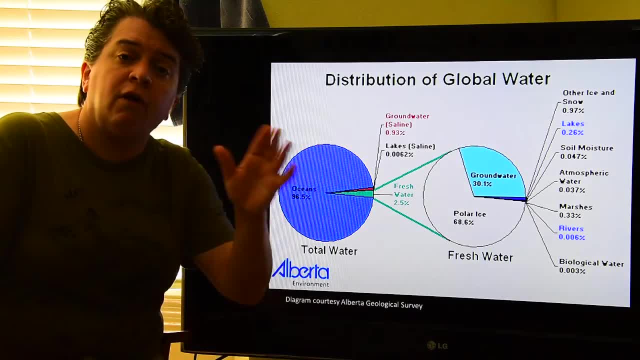 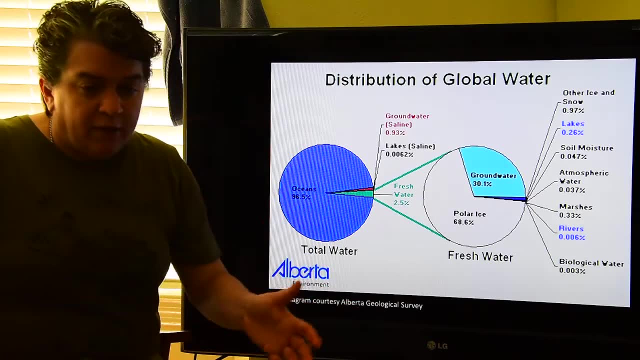 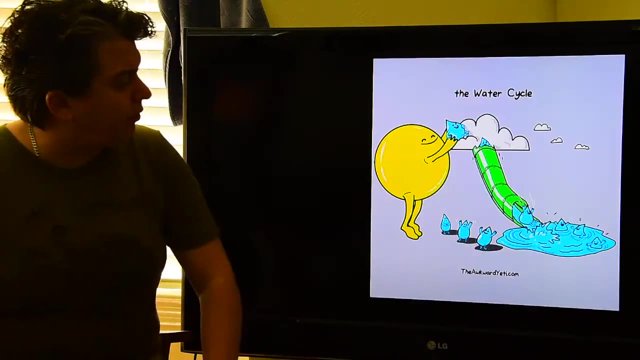 All of the water molecules on Earth are slowly moving around, So we might have some water molecules in the ocean, but they'll get evaporated and go into the atmosphere and then they'll fall as rain and enter a river, something like that. 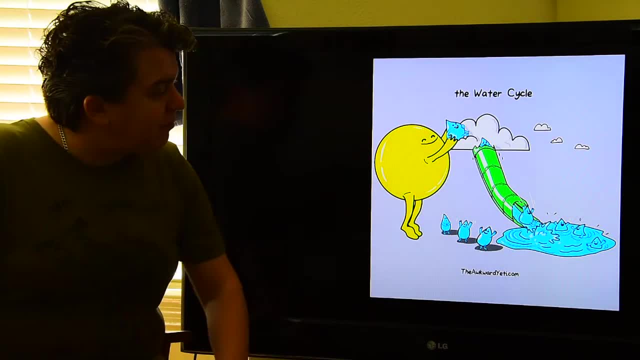 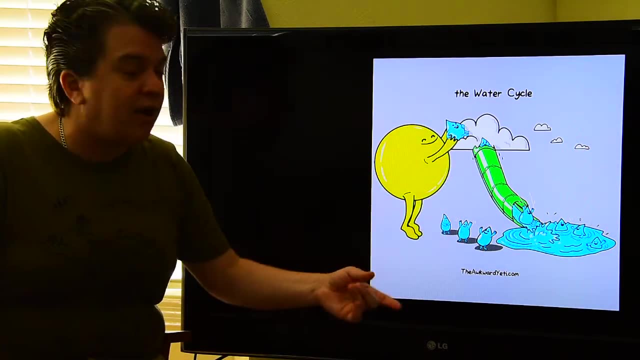 And we call this the water cycle, And this is just a really cute way of showing the water cycle, where we have the sun picking up the water, putting it in the sky. I just mostly use this diagram because I love the website name. 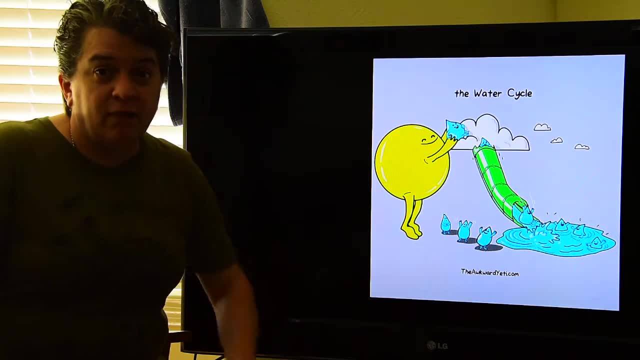 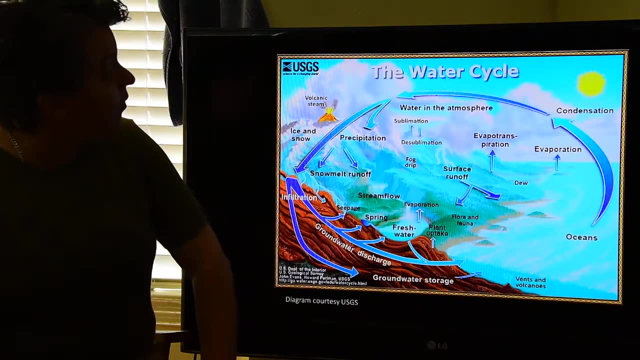 It's called the Awkward Yeti. I guess you know even yetis can be awkward at times. No, in all seriousness, this is a much better diagram of the water cycle. This comes from the United States Geological Survey. 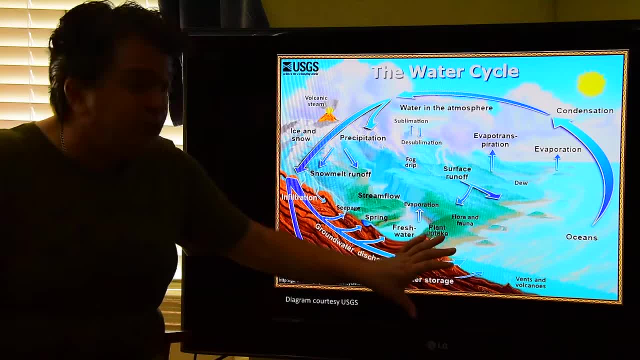 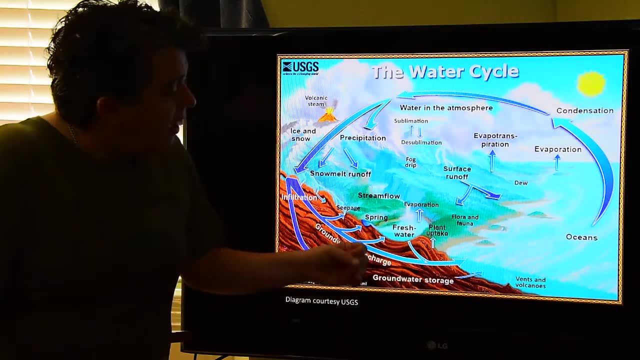 And it really just shows all the different places on the planet water is located and how it ends up moving between those places. And no, I don't expect you to memorize it, I don't expect you to memorize every little detail of here. 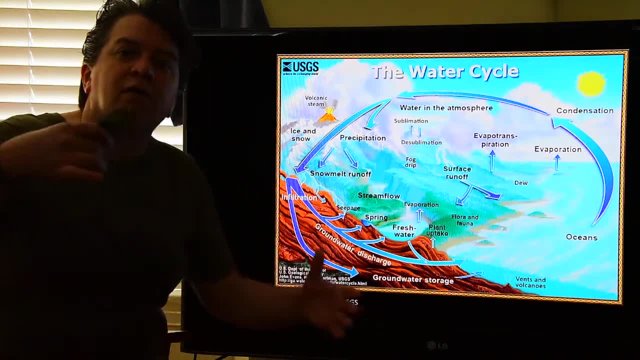 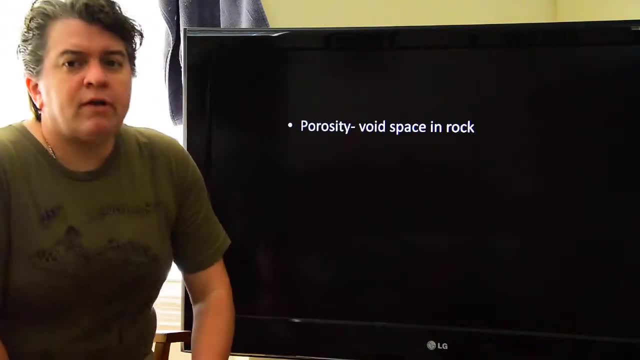 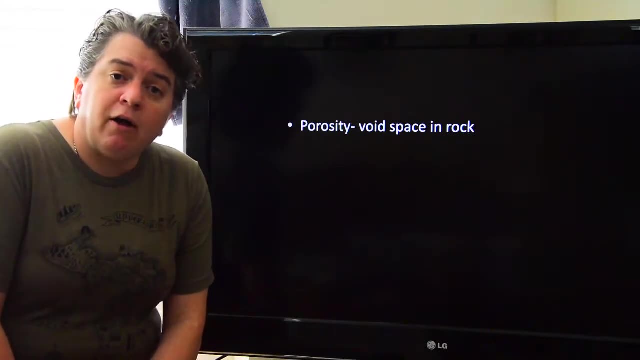 But you do need to recognize that water is in constant motion around our planet. So when we start looking at water resources and the water that people use on the planet, we're going to use a lot of that groundwater for different things: for drinking water, for industry, for irrigation. 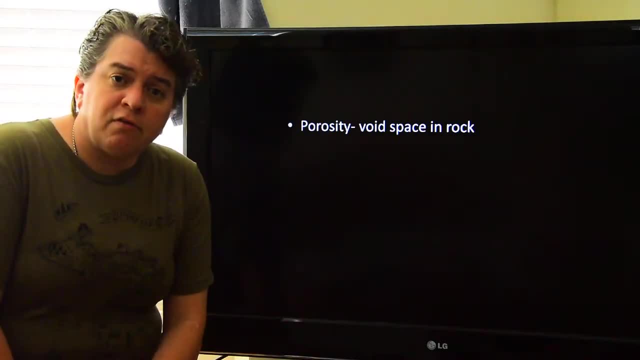 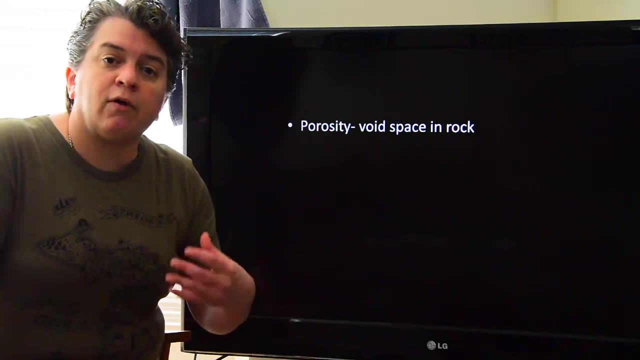 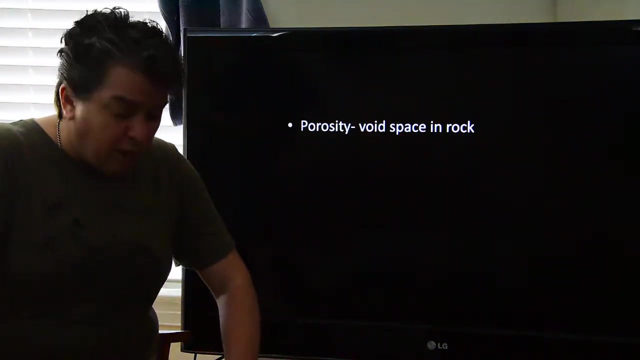 And so it becomes quite important that we start understanding how groundwater behaves, And to do that, we have to look at the rock or sediment that the groundwater is inside, And when we're describing some of this rock or sediment that holds the groundwater, one of the descriptions we use is porosity. 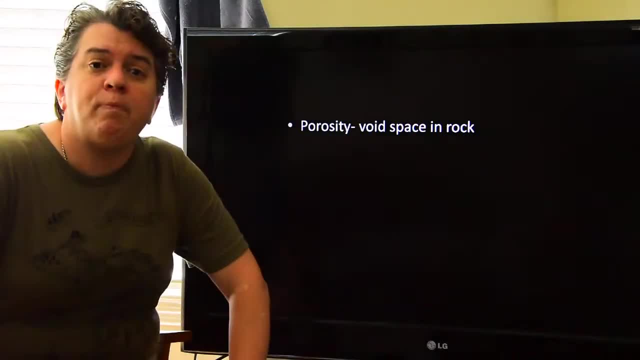 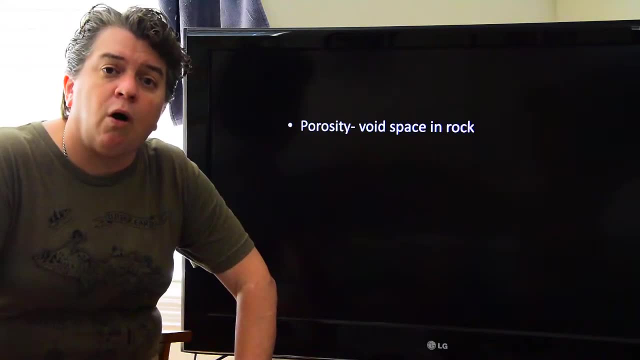 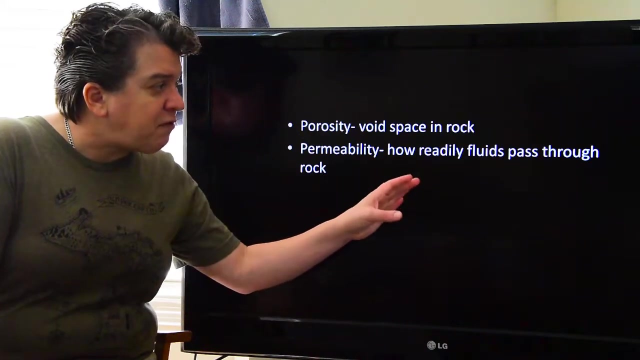 Porosity is void space in rock or basically open space, And that is important because we need open space in our rock or sediment to hold water. And then we also have this characteristic called permeability, And this is how readily fluids flow through a rock. 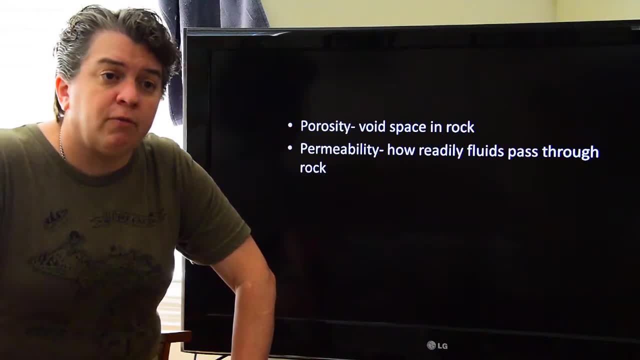 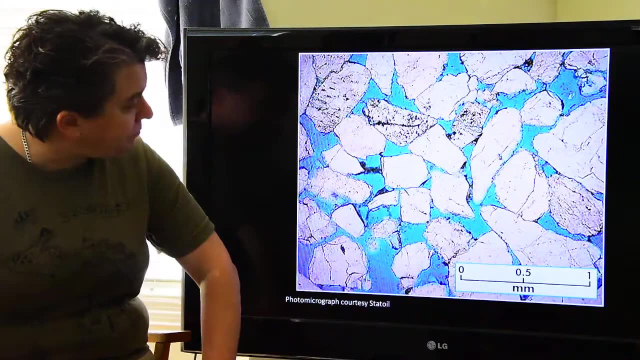 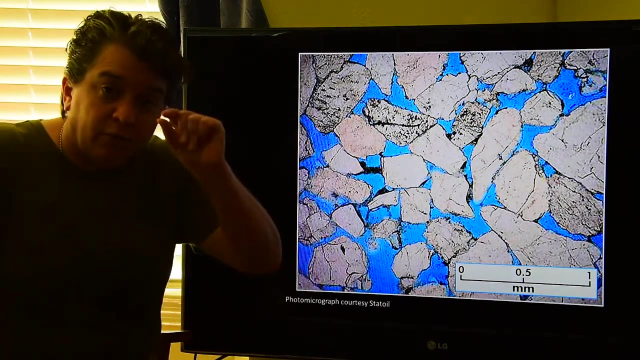 And you want things to be able to flow through the rock, because if you drill a well, you want the water to be able to flow out of the rock into your well. So if we look at this, this is a thin section. It's where we cut a rock really, really thin. 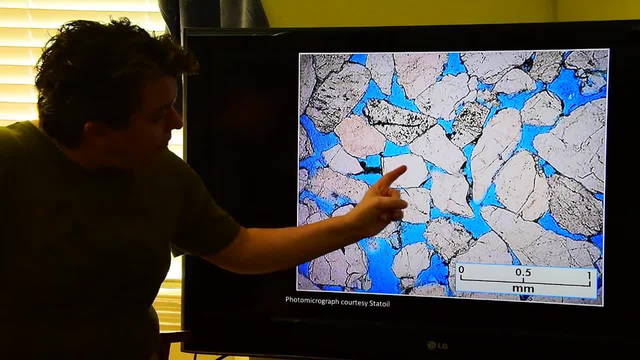 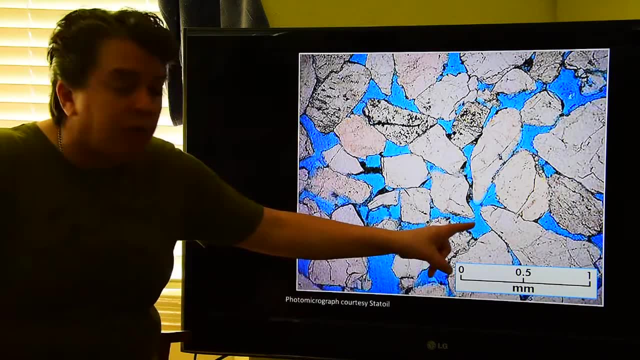 We stick it under a microscope and we look at it And every single one of these little white areas that is a grain of sand And this blue area is porosity. That's the open space. So this would be a rock that has a good amount of open space. 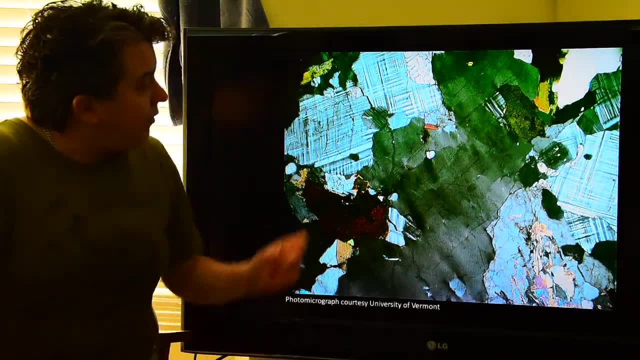 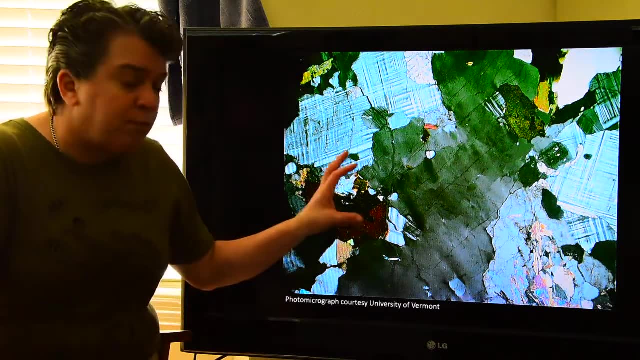 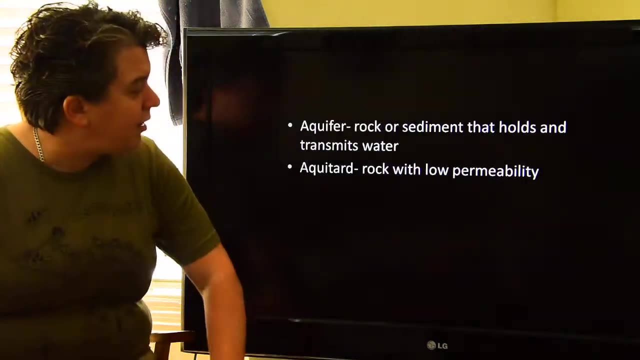 so it could hold a lot of water in it. These are all bits of quartz, but you don't see a whole lot of that blue in this one, So this would be a rock that could not hold a lot of water because it does not have a lot of porosity. 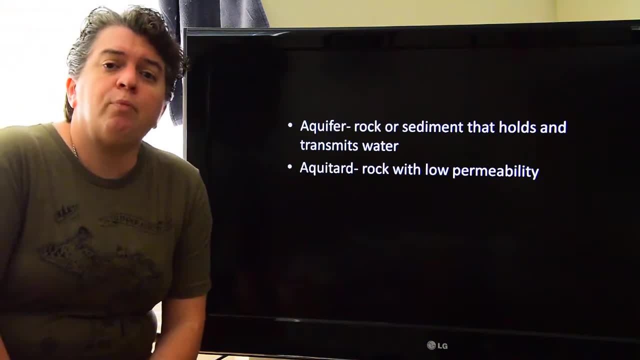 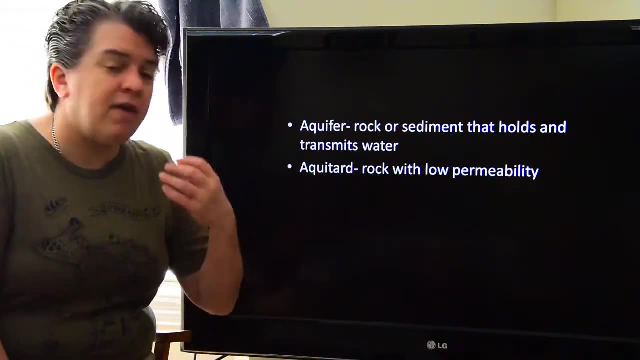 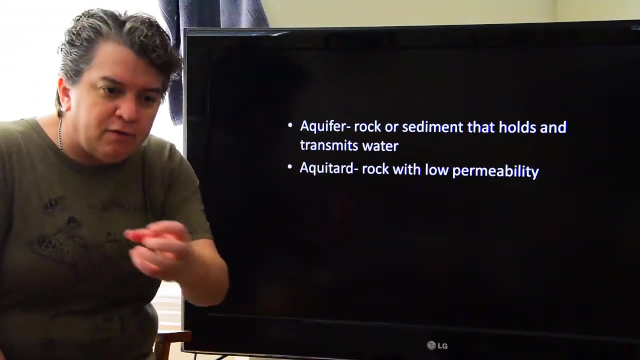 So ultimately we get two basic sorts of rocks. underground We might have an aquifer, which is rock or sediment that holds and transmits water. It has a lot of porosity, That's the holding it And it allows that water to flow through it. 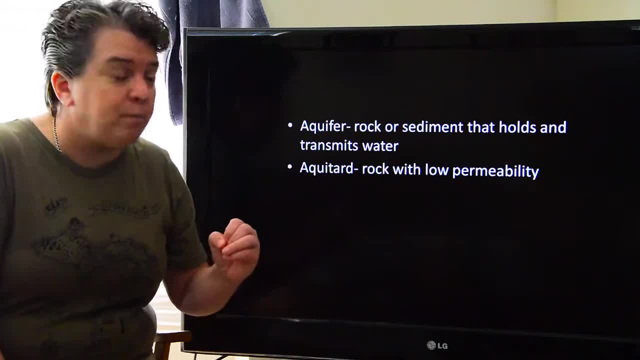 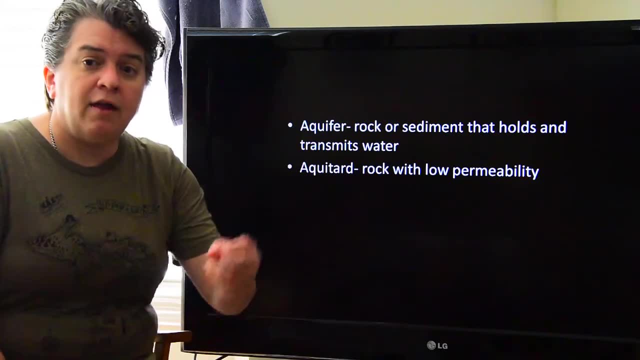 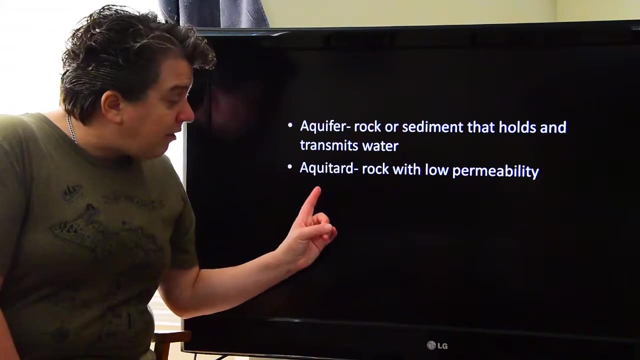 That's the transmitting water, That's the permeability. So an aquifer has good porosity, good permeability. It holds a lot of water for us, And then the water easily flows into wells, if we drill into them. We also, though, could have an aquitard. 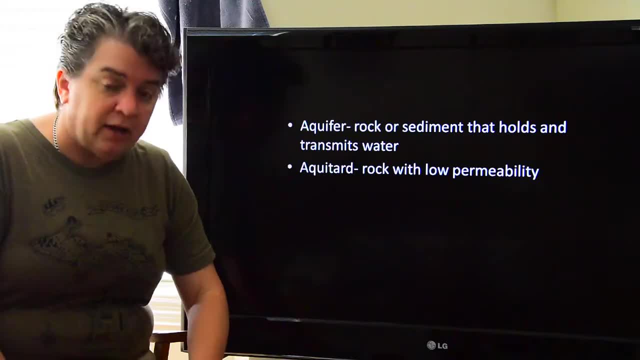 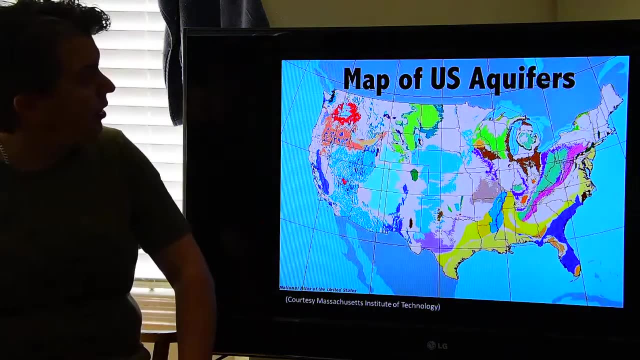 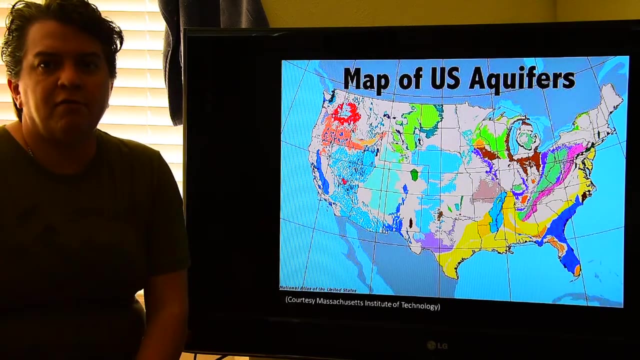 An aquitard is a rock with low permeability, So it prevents water from flowing through it. Now, this is a map of some of the main US aquifers, But I want you to realize that these are not the only aquifers. 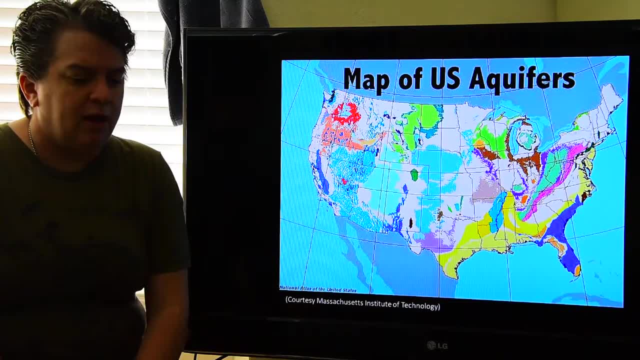 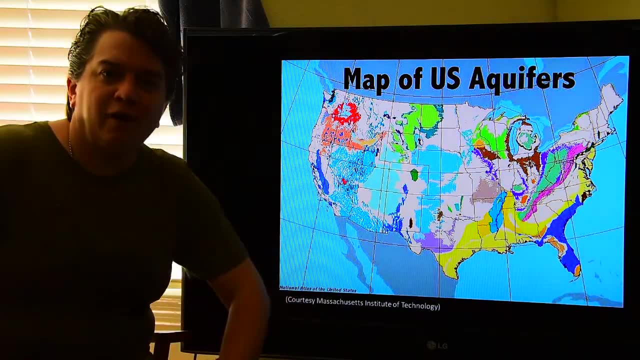 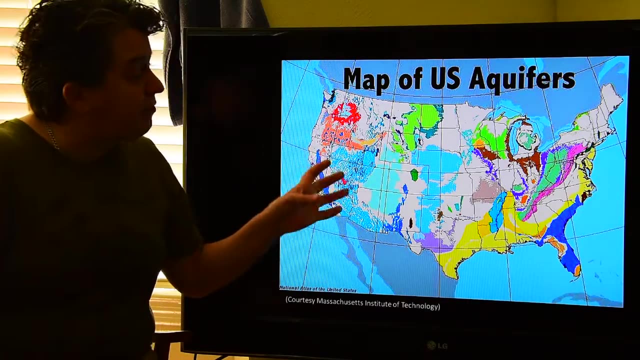 that exist in a location, And so, anyway, yeah, these. sorry I'm doing this at home and sometimes my cats are misbehaving, So oh well, Anyway, this is a map of some of the major US aquifers. 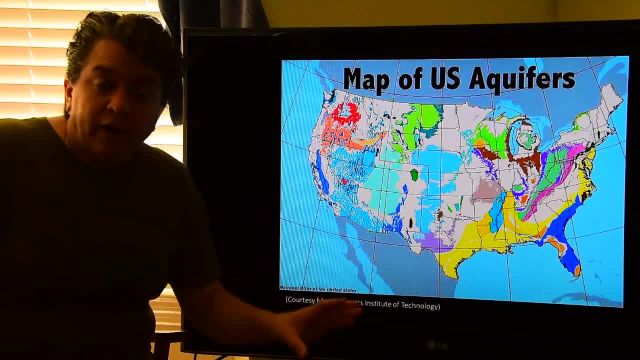 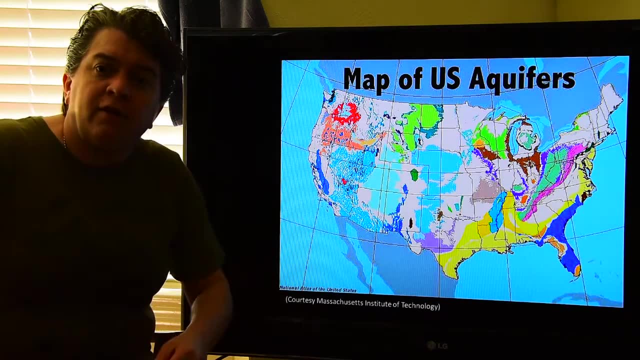 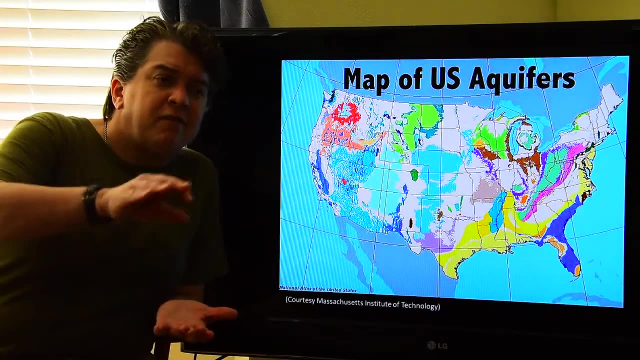 These are not the only aquifers that exist in those places. Just realize: the rocks underneath our feet in many places are very much like the Grand Canyon. right, You've seen. if you haven't visited the Grand Canyon, you've at least seen it. 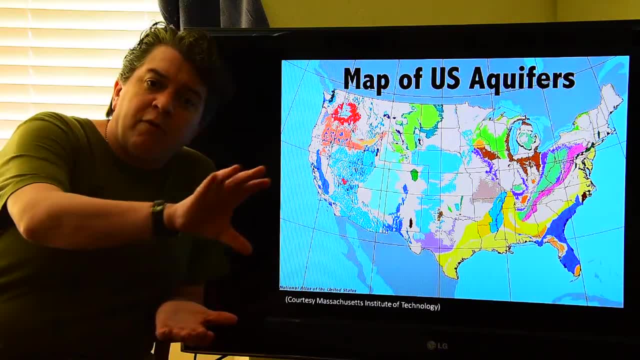 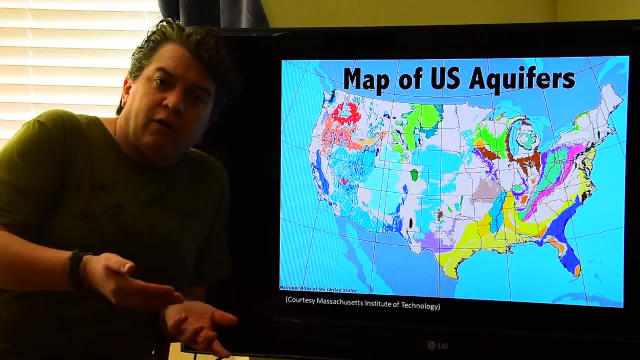 where there's all these different layers. And now imagine some of those layers are aquifers and some of those layers are aquitards. So it's actually when we look at groundwater behavior in the subsurface, it can be kind of complex. 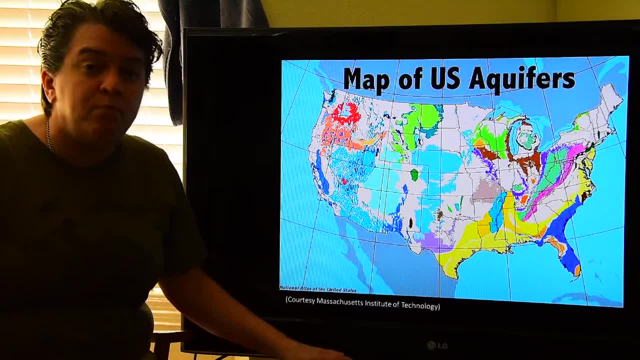 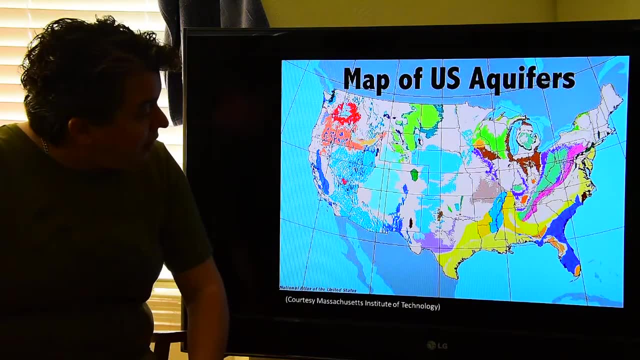 But what we've done on this map, we've looked at big, important, major aquifers And so you can see some of the different ones underlaying parts of the US And there's, like the Edwards Aquifer here in Texas. 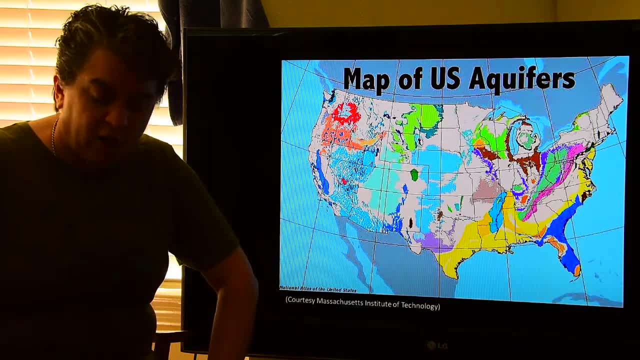 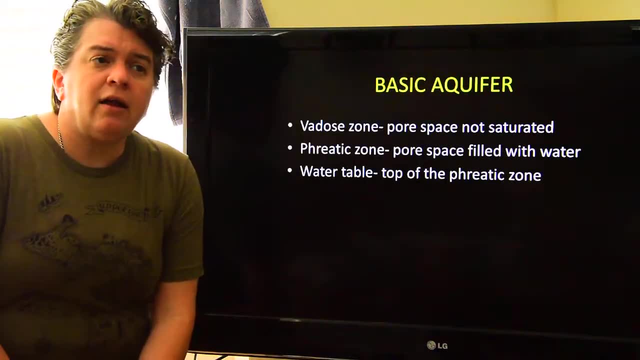 This is the Ogallala Aquifer, which is very important for agriculture in the Great Plains, And then, of course, there's many other ones there. So let's look at one of these very basic aquifers. These aquifers have parts to them. 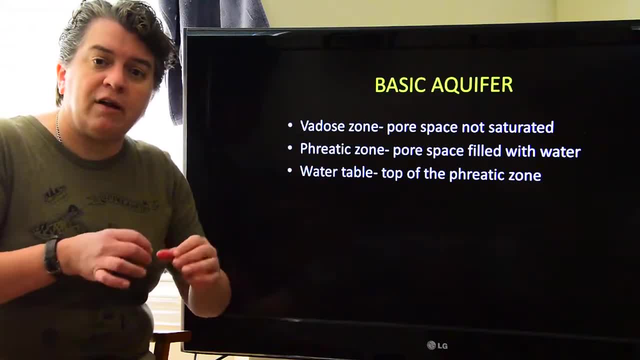 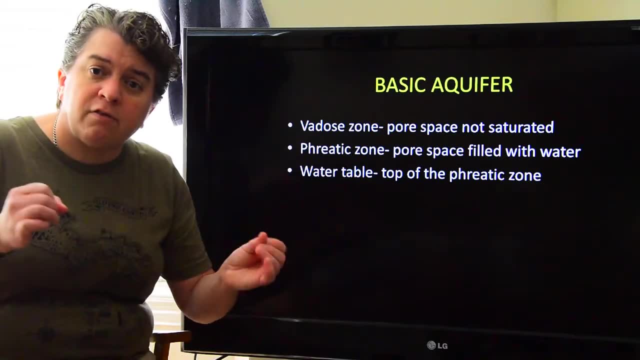 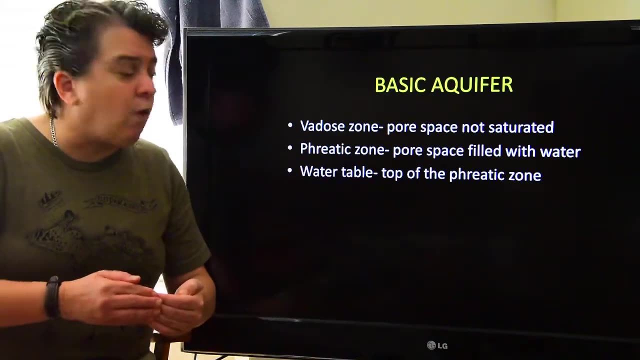 There's the Vados Zone, where the porosity is not saturated with water. We're not saying that there's no water in there. There might be a few droplets and things stuck to different minerals and sand grains, but it's not 100% filled with water. 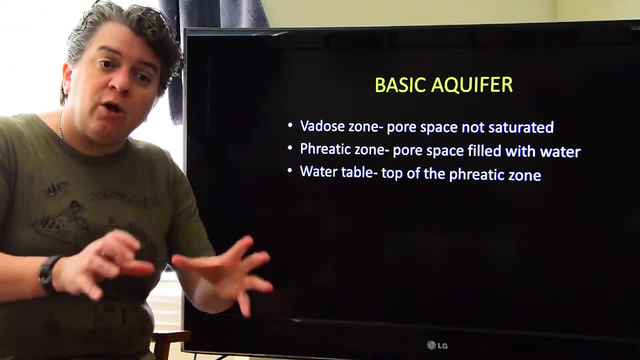 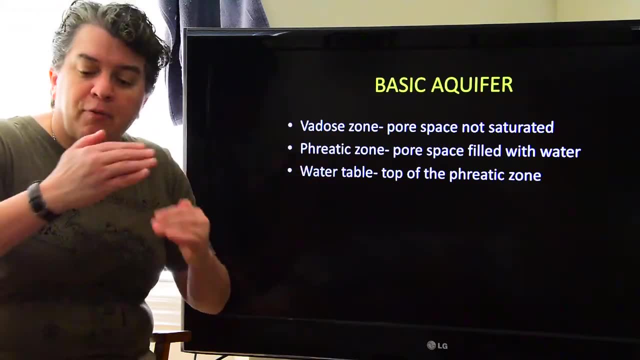 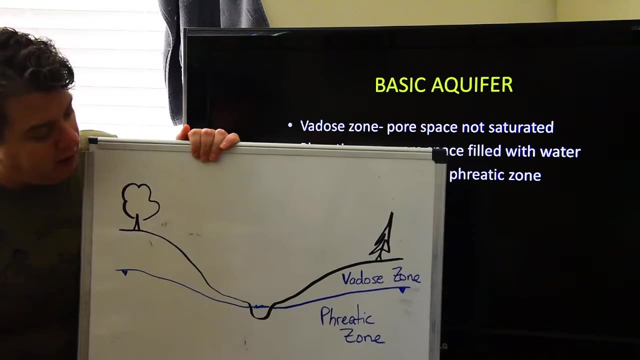 Now the area that's 100% filled with water is called the phreatic zone, And the water table separates these two. So right here I have a very basic drawing of a cross-section of an aquifer. So here's Earth's surface. 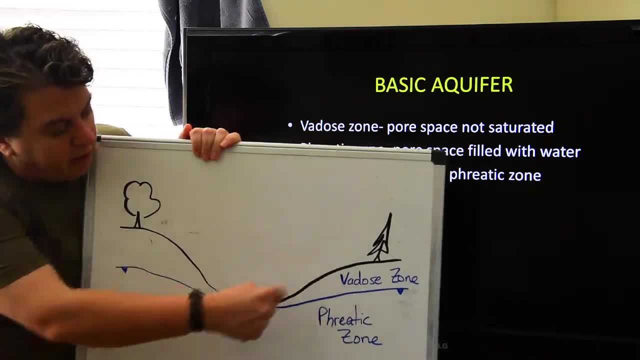 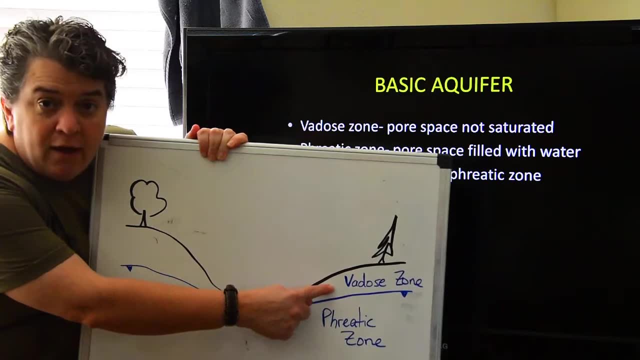 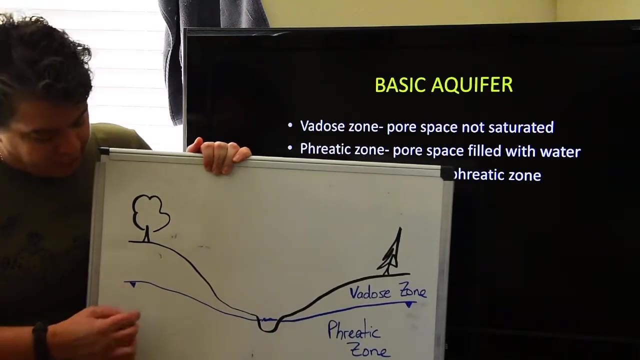 Here's a little pond or maybe a stream And this line here. that is the water table that separates the Vados Zone from the phreatic zone. When we draw these on a cross-section, we show the water table with a little triangle on it. 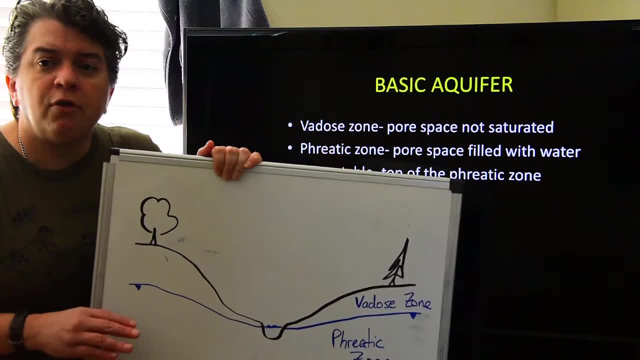 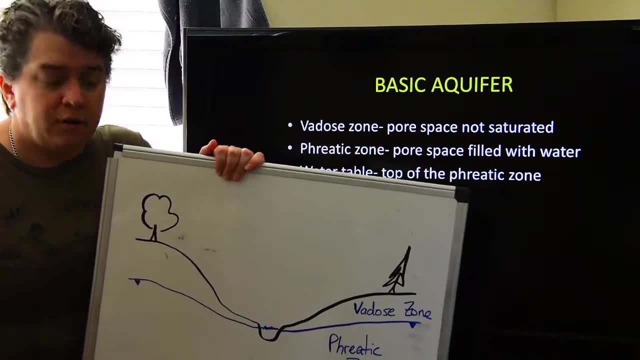 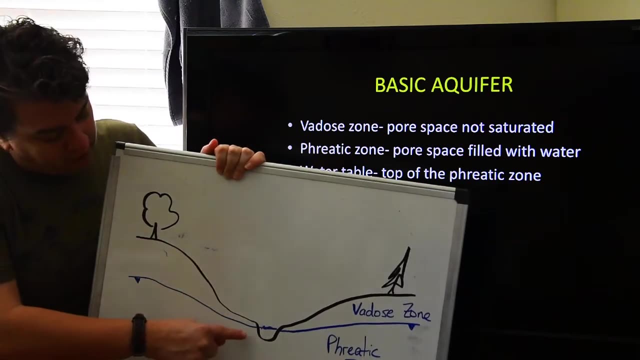 And that's to show that we're drawing the water table and not just a different layer of rock, And a couple of things to notice about the way this is drawn. When we have a hill on Earth's surface, we also have a hill in the aquifer. 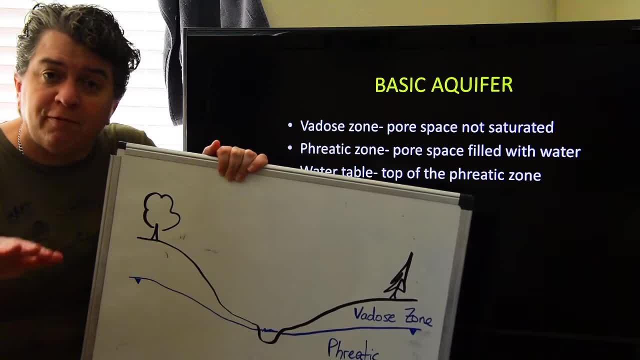 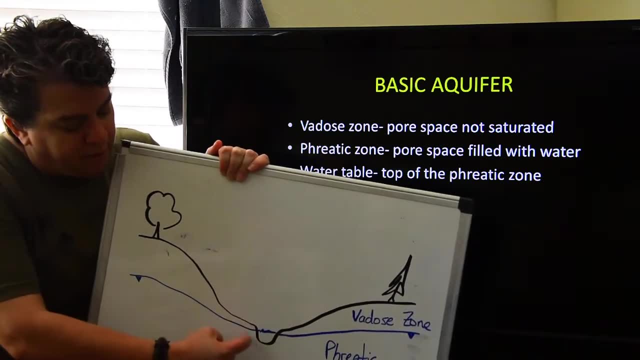 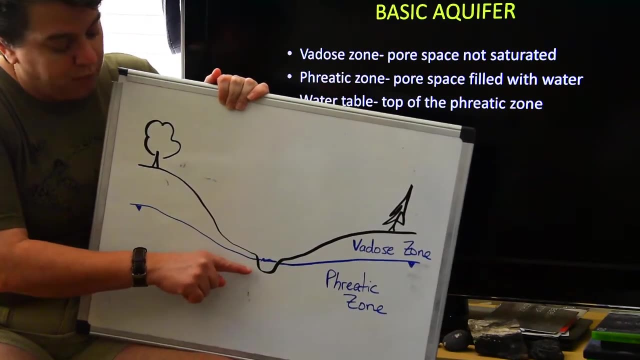 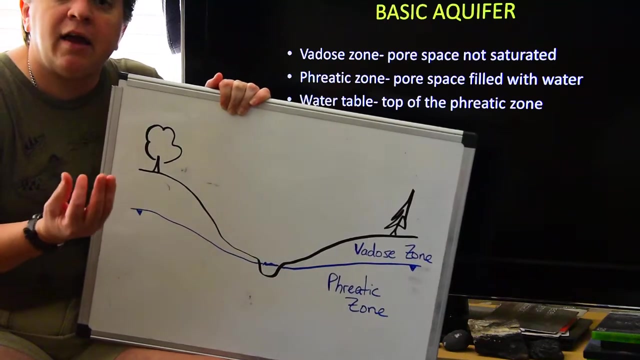 So the water table is not flat. It has topography. It has ups and downs to it. Also, wherever we have surface water, like this little pond, that's a place where the water table intersects Earth's surface. So if you see any standing water, 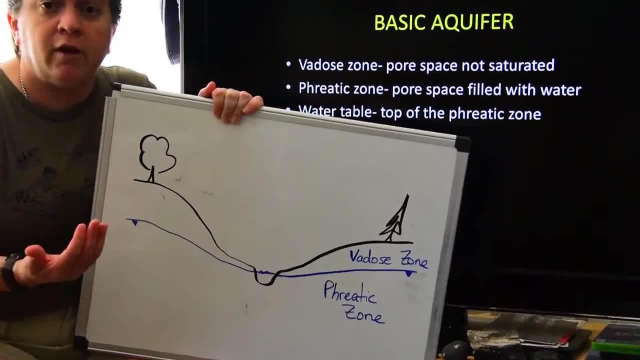 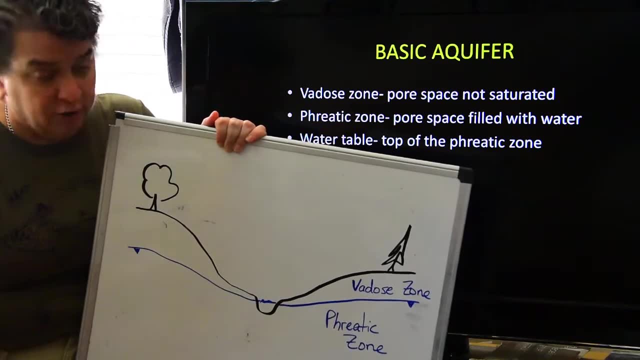 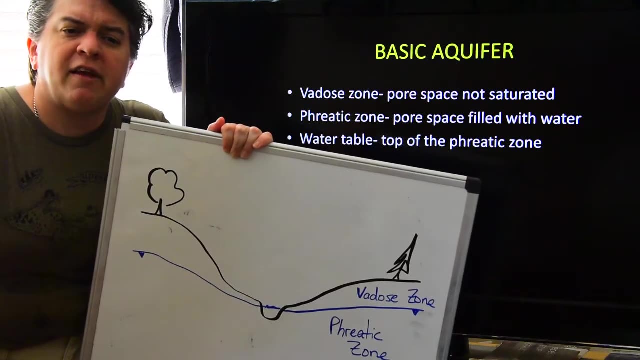 a pond or a spring or a stream or a swamp. that tells you the water table intersects Earth's surface at that location. I also want you to realize that sometimes people think of aquifers as just like giant lakes underground. Well, they're not really like that. 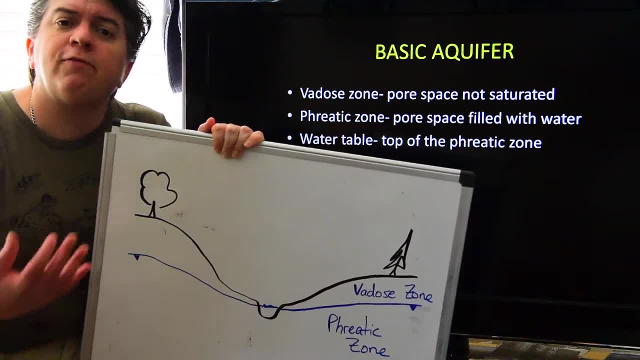 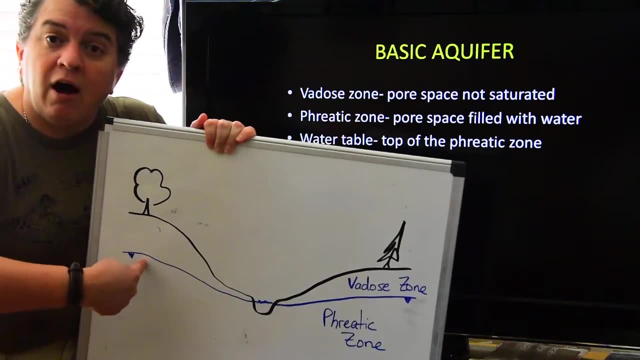 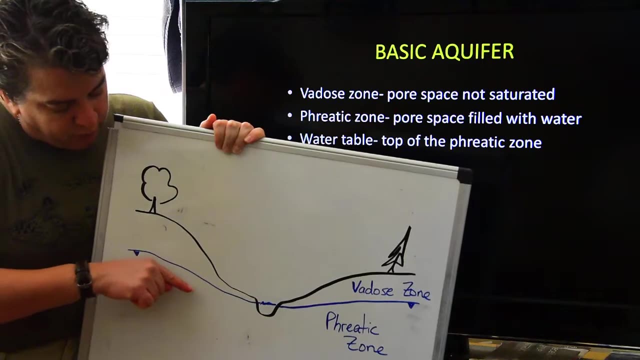 They're more like a river underground. They are flowing. The water in the aquifer is moving, And how does it move? Well, it moves from higher elevation to lower elevation, just like water moves on Earth's surface, And so this water would be flowing in that direction. 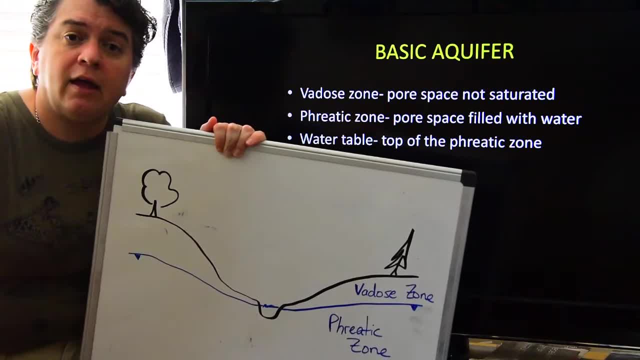 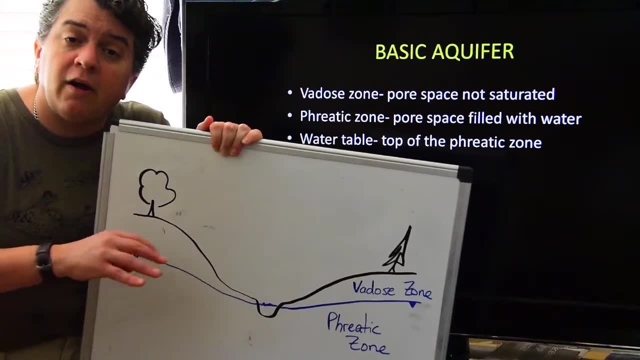 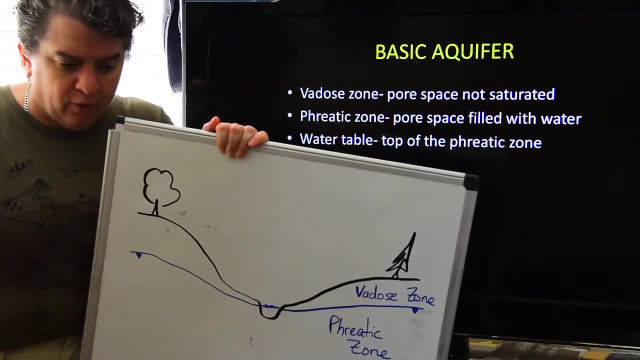 And that becomes important when we start looking at groundwater contamination, because that contamination is not just going to sit there, It's going to move around underground And it can get kind of complex because this stuff- unlike in a river, where it just flows in the channel- 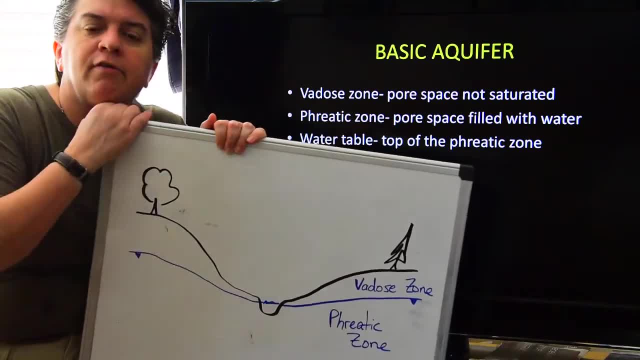 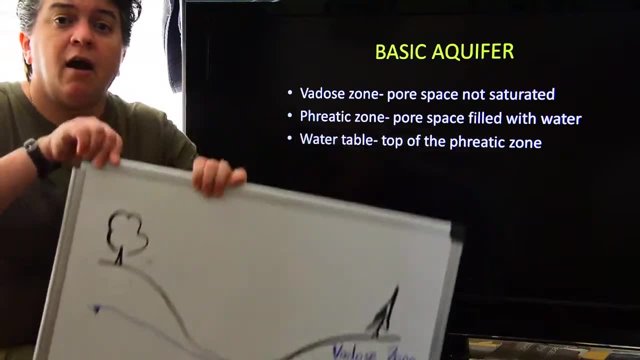 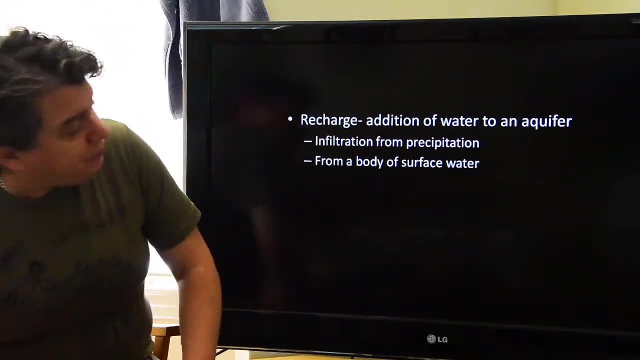 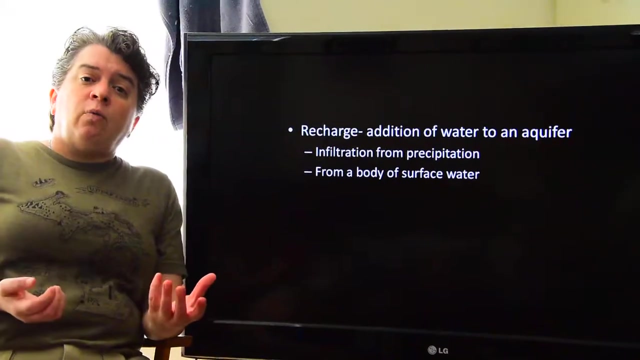 it has to find its way in between all those little sand and sediment grains. So, anyway, that's kind of a very, very basic aquifer. Now, when we're dealing with aquifers, water is being added to aquifers and it's also being taken away from aquifers. 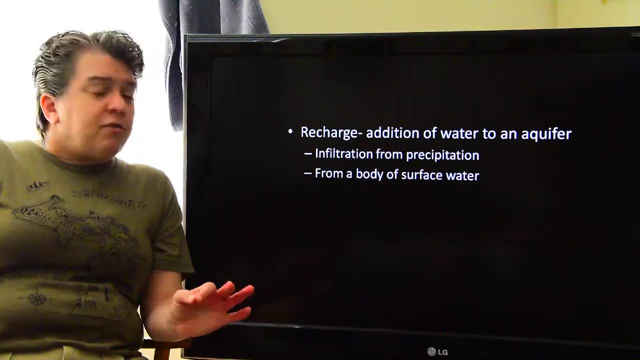 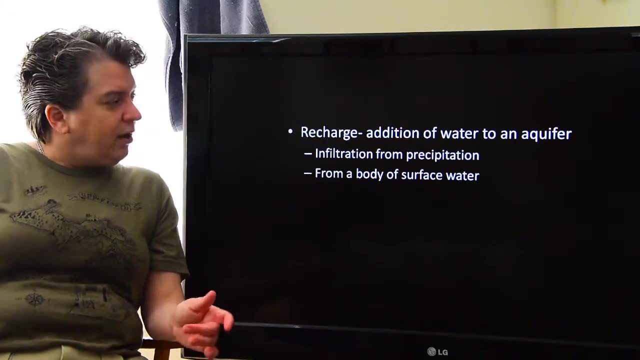 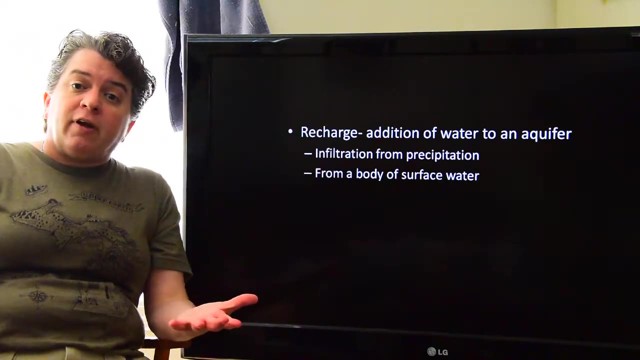 The addition of water to an aquifer is called recharge, Sort of like recharging a battery, right? You're adding a charge to it, So, anyway, recharge is adding water to an aquifer, And this could be from infiltration, from precipitation, right. It rains on the surface and some of that rainwater seeps into the ground and will join the aquifer. Or it could be from a body of surface water. You could have a pond or a river that's actually allowing water to seep out of it into the ground. 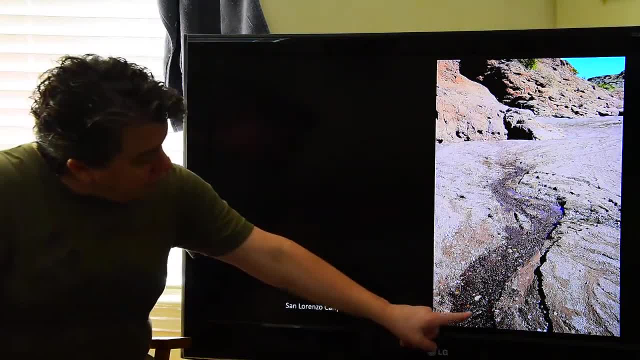 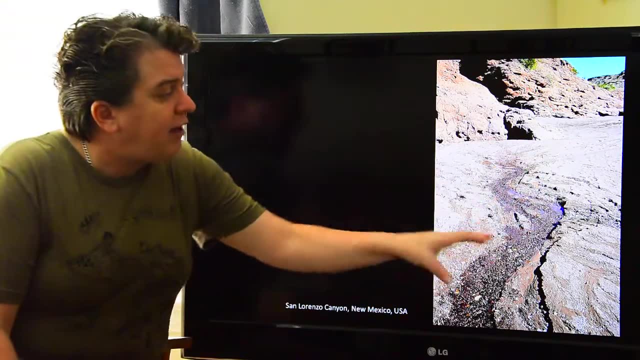 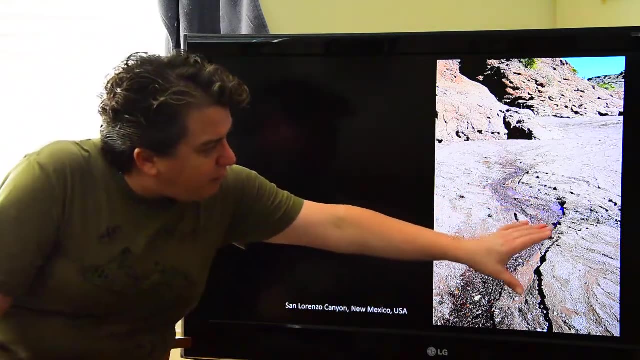 And that's actually what we're seeing right here. Right here, we have water and then it basically disappears. All of this sand over here is dry, And that's not because the water- just you know- miraculously- is gone. What's happening there? the water is seeping into the ground. 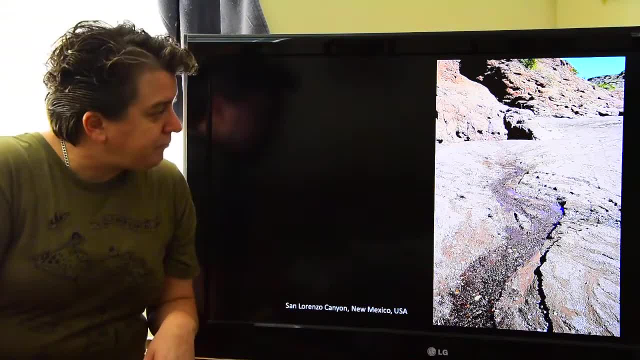 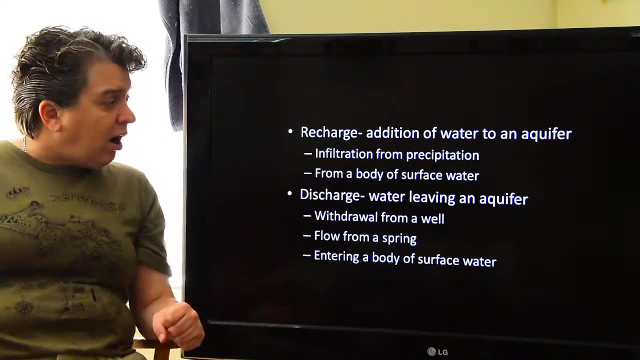 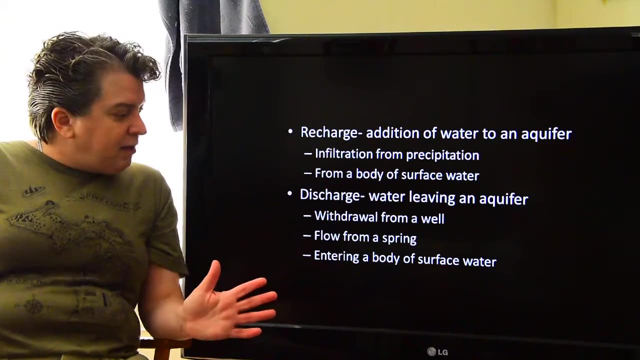 and it's becoming part of the groundwater. Now, just like I said, water can be added, Water can be taken away from an aquifer And that is discharge- Discharge water leaving an aquifer, And this can be, this can be natural. 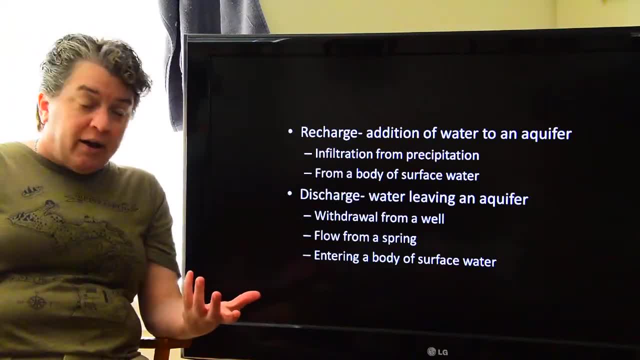 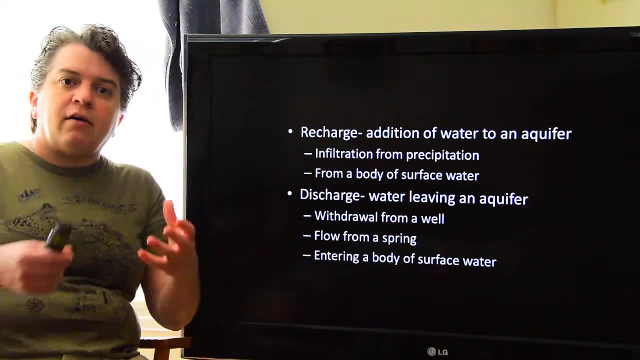 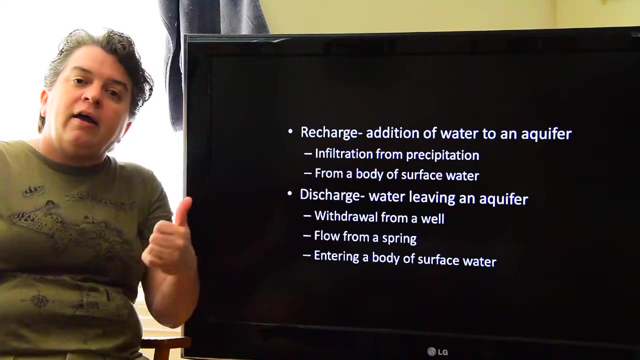 It could be water coming out of a spring. It could be water entering a body of surface water. So, instead of like a stream, giving water to the surface water, the aquifer, maybe the aquifer is feeding water into a pond or into a body of surface water. 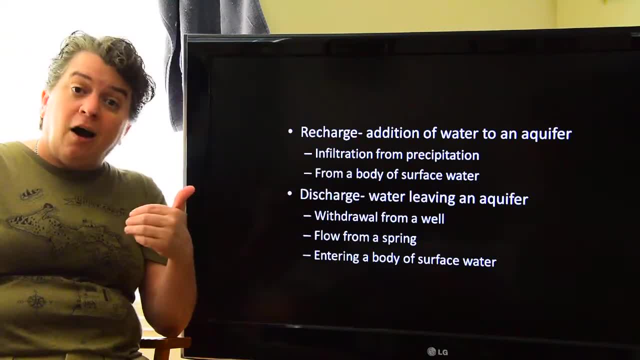 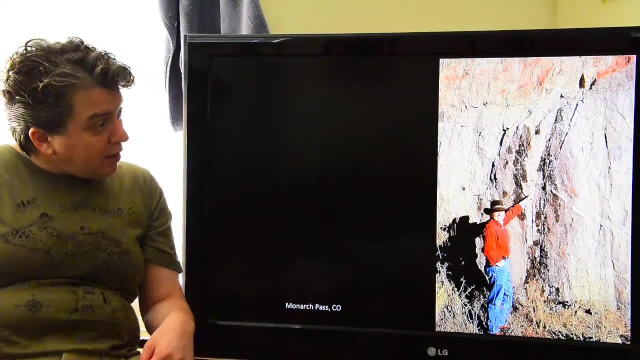 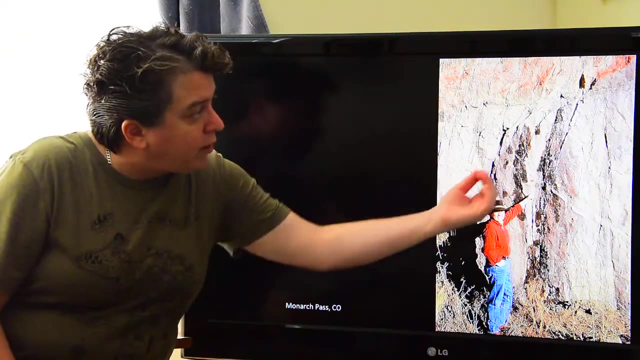 Or discharge can be caused by us. We can drill a well and then extract that water out of the aquifer. So what we're looking at here, this is basically a spring. See those darker areas there. That's where water is actually coming out of this rock. 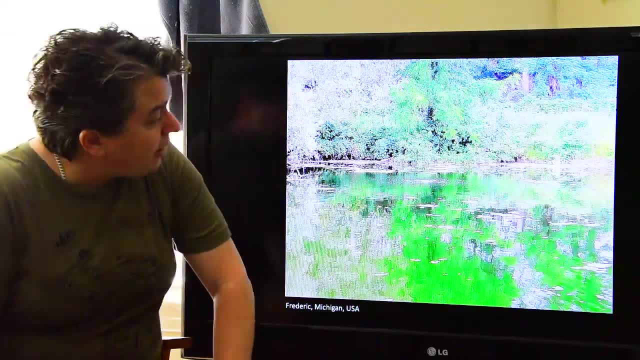 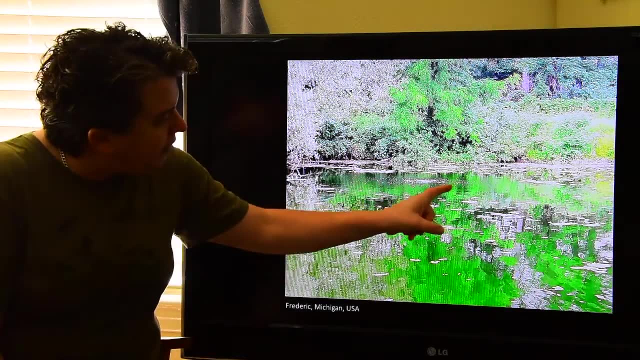 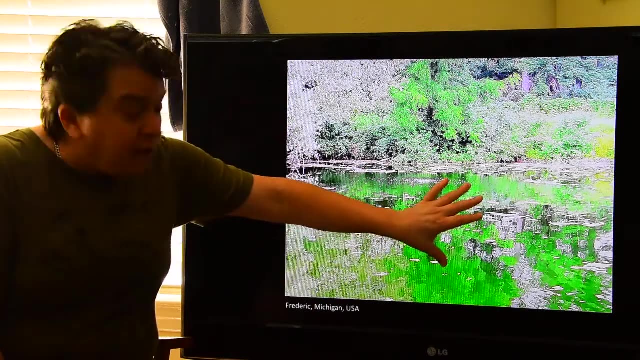 along some cracks. This is a nice little pond and it is a spring-fed pond- This area here where it looks kind of bubbly. there's a spring underneath this where the groundwater is bubbling out and feeding water to this pond, So that's discharge out of the aquifer. 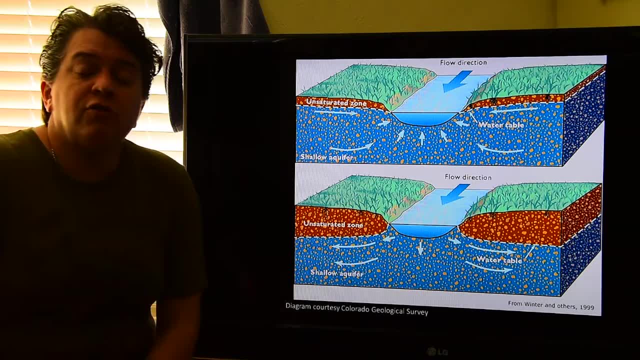 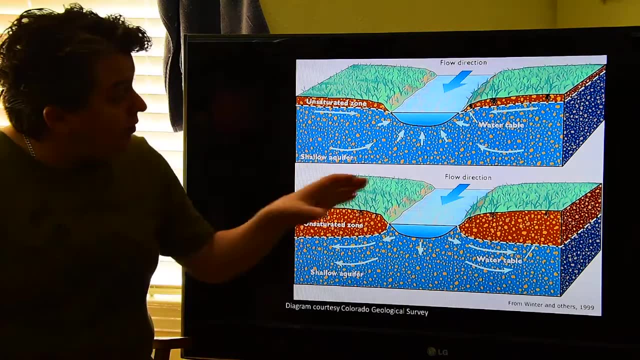 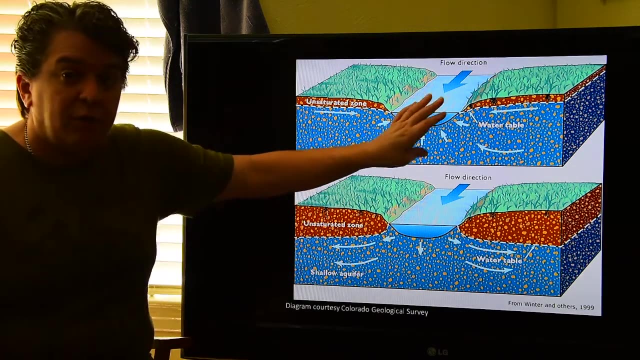 into that surface water, And I mentioned rivers can sometimes either gain or lose water to an aquifer, And this one right up here this is called a gaining stream. This is where the water table, the aquifer, is actually giving water to the stream. 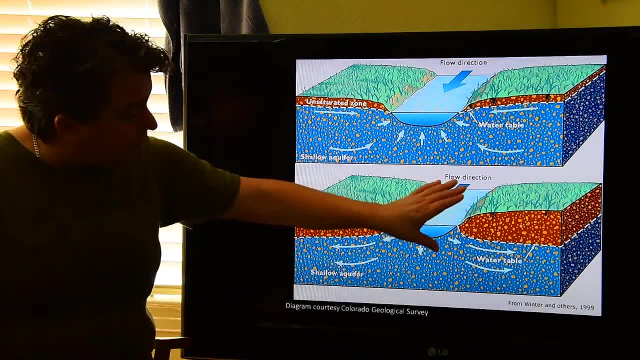 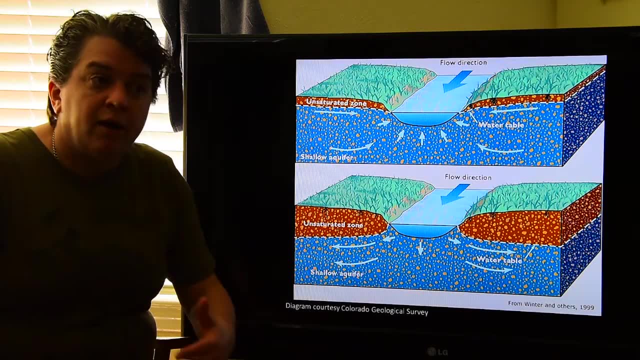 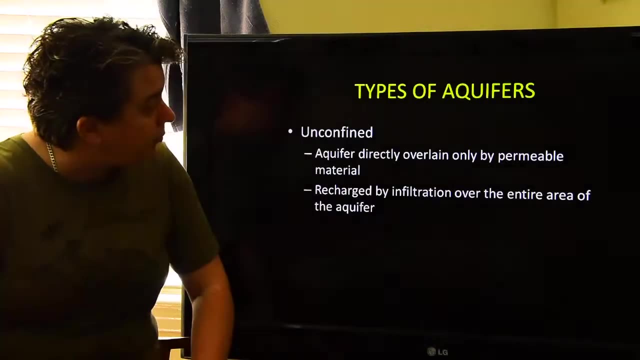 This is called a losing stream. This is where the stream is giving the aquifer water And those. depending on where you're located and the rock types and the climate, you can have gaining or losing streams. Now there are different types of aquifers. 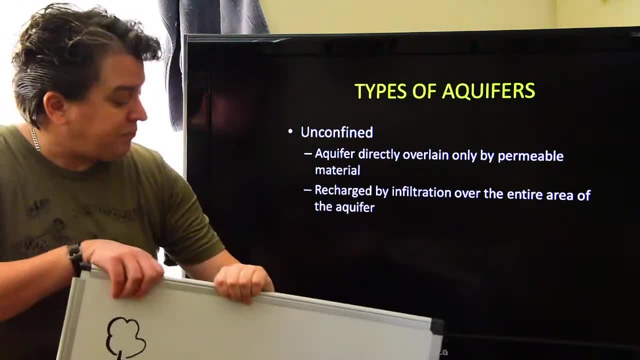 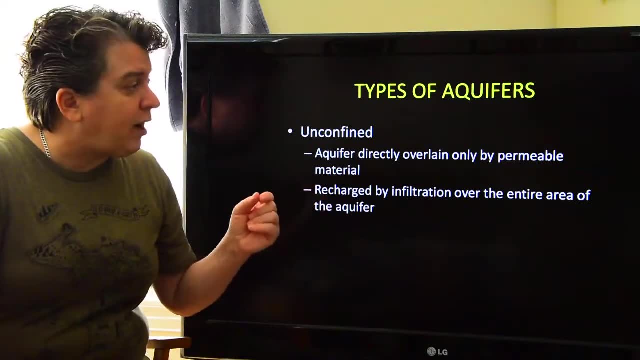 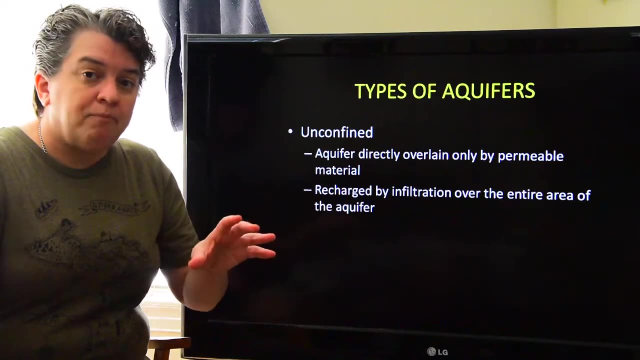 that exist on Earth. First of all, I have this thing called an unconfined aquifer, And here the aquifer is directly overlaid only by permeable material, So there's water can pass through all of the material over the aquifer. 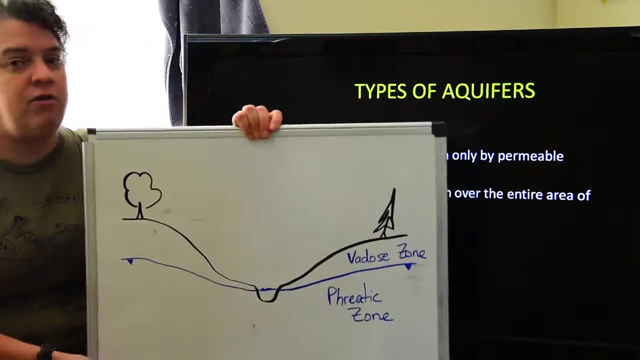 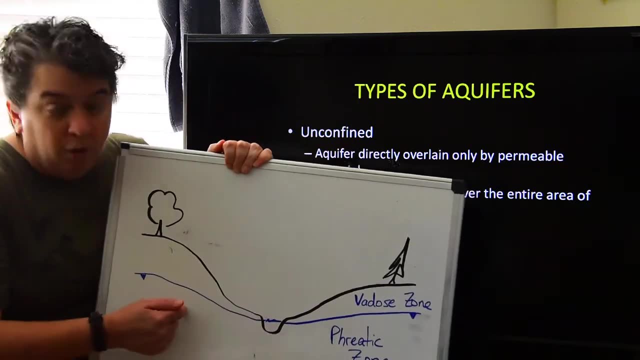 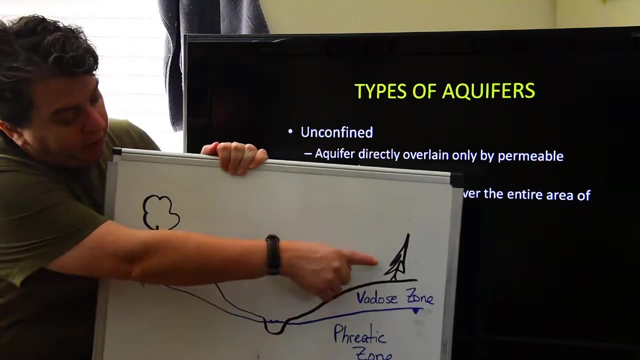 So this is going to be recharged by infiltration over the entire aquifer And that's like what I had drawn here. Everywhere above the water table is permeable material, So it doesn't matter if it rains here or it rains over there. 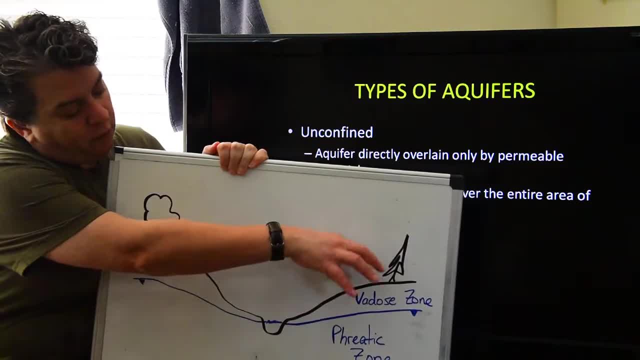 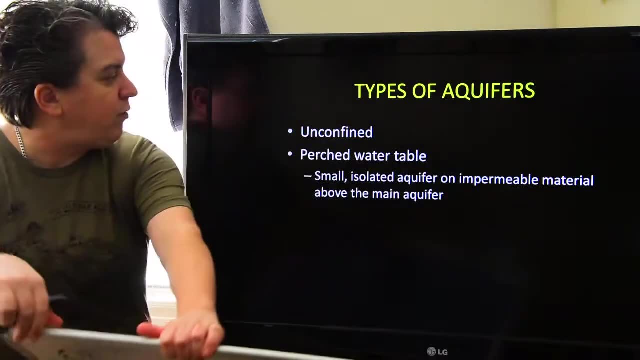 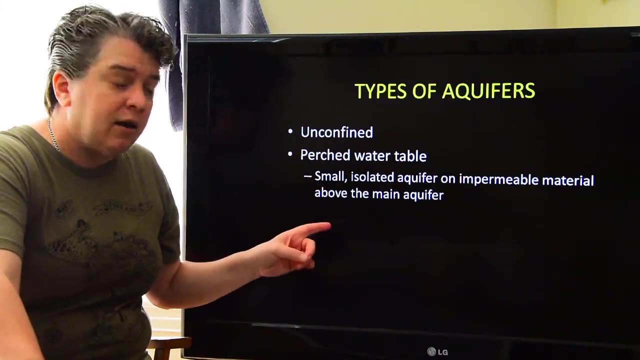 Some of that infiltration from the rainfall will seep into the ground and join the aquifer. Now this is going to be different from what we call a purging stream. This is going to be a perched water table. A perched water table is a small, isolated aquifer. 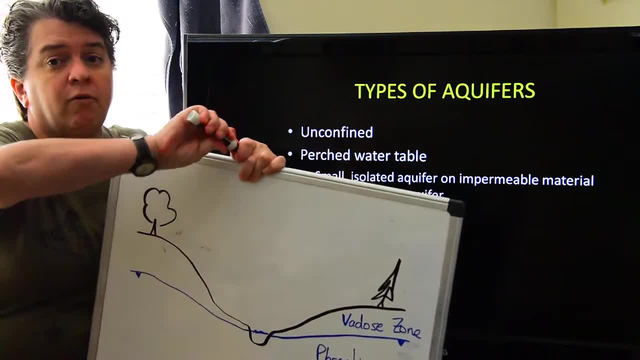 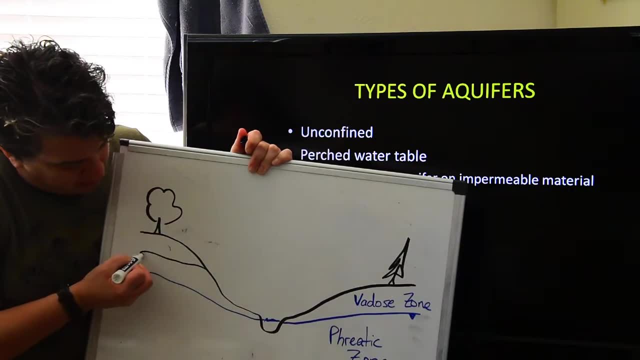 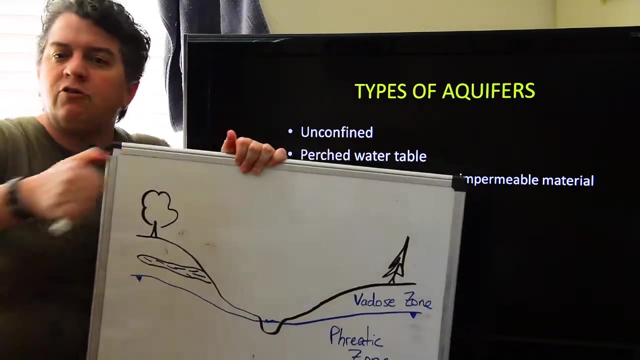 on impermeable material above the main aquifer. So let's say this is my main aquifer down there. But maybe we have a layer of impermeable rock here. Something like shale. Shale is very commonly impermeable. If it rains in this area, then 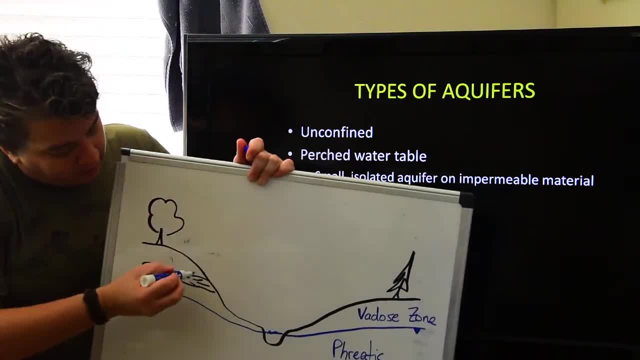 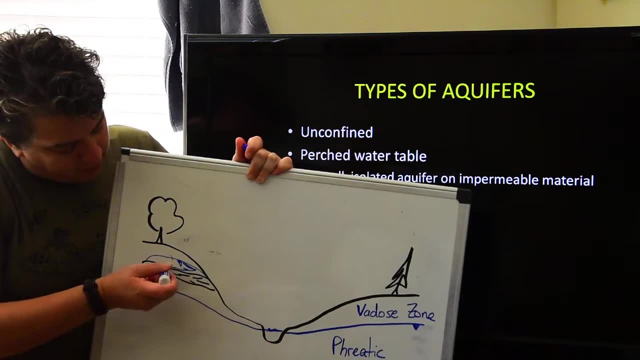 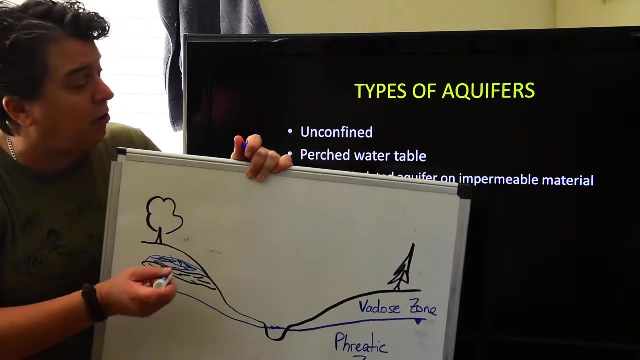 the water is going to infiltrate and it's going to get stuck on top of this shale. It's going to get stuck here, So we'll have this area right here of saturated sediment sitting on top of that impermeable shale. That's a perched water table. 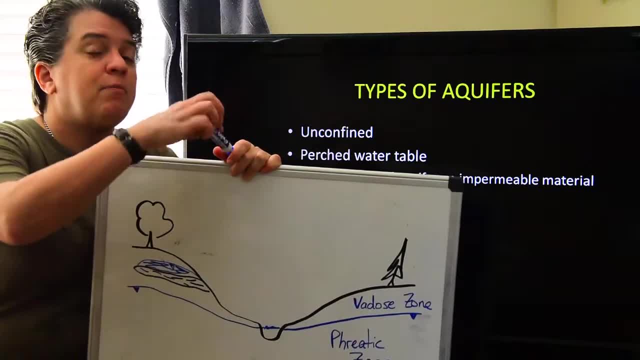 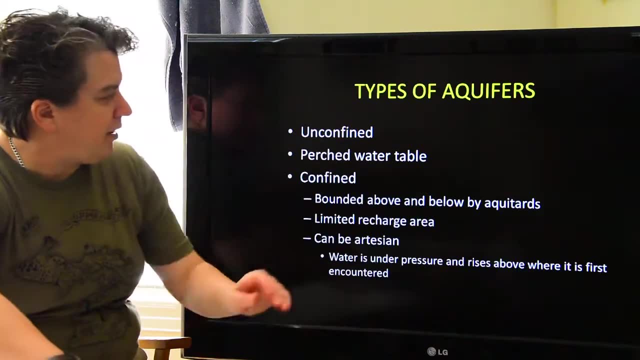 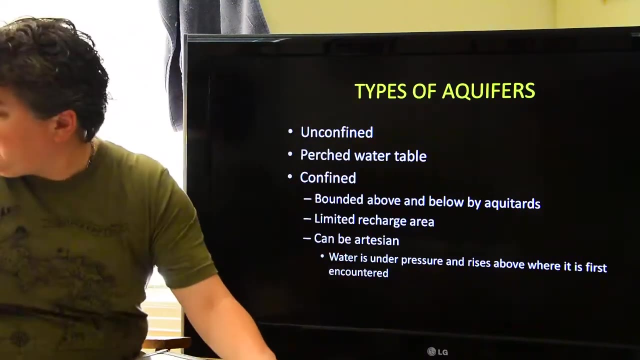 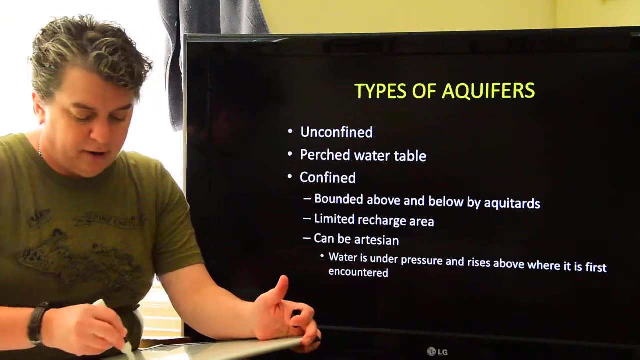 So they're small, but they're above that main regional aquifer. Now our next type of aquifer is called a confined aquifer, And to have a confined aquifer you need impermeable material above and below the aquifer unit. 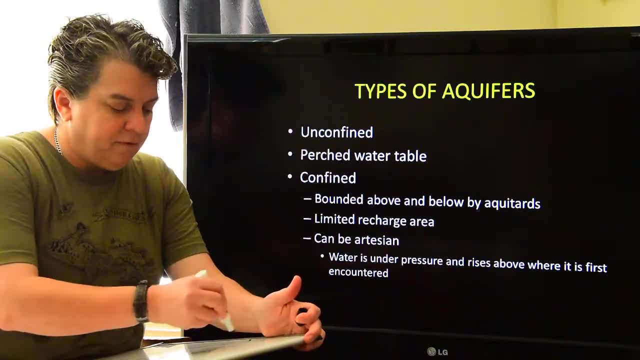 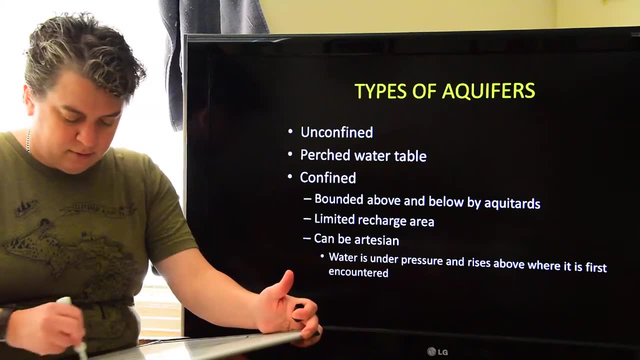 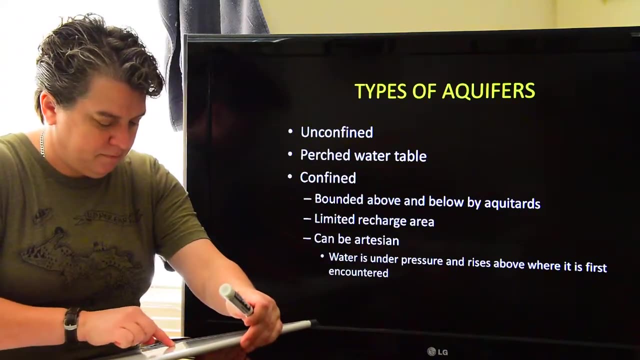 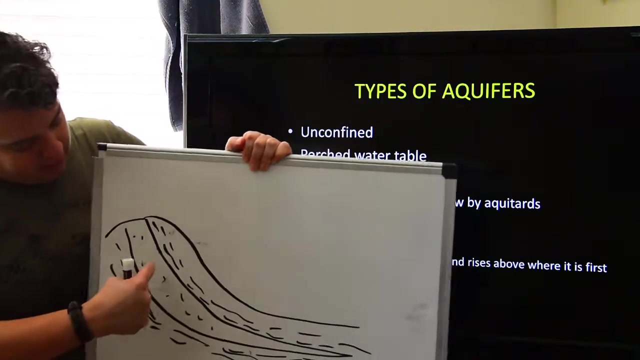 So I'm going to draw in a confined aquifer here And I'm doing it nice and fast. Okay, So let's say what we have here is our aquifer. That's going to be something like sandstone. Sandstone is great for an aquifer. 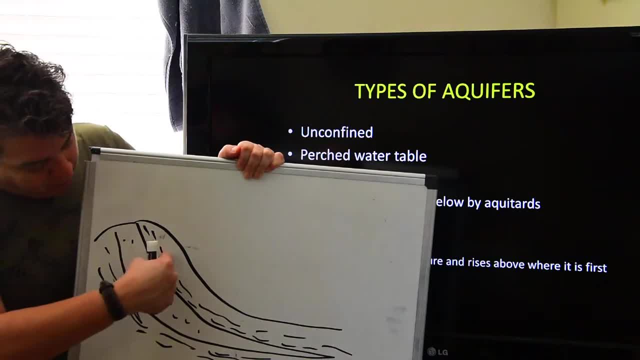 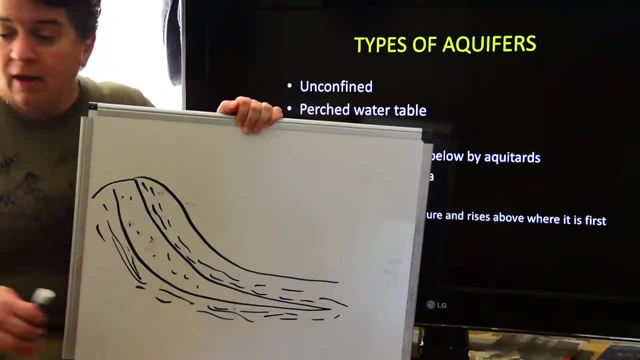 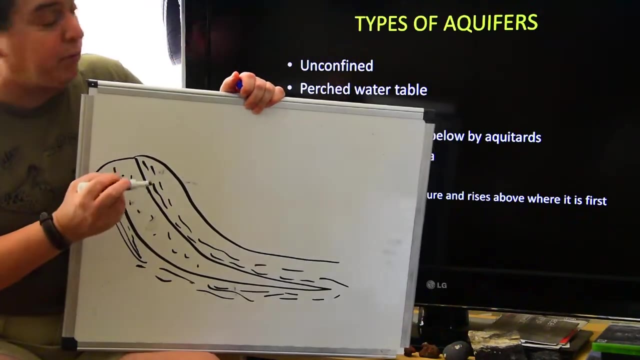 because it has lots of porosity and permeability. Above and below that sandstone is some of that impermeable shale that we have Now this confined aquifer right. it's confined by the impermeable material. This is going to have a limited recharge area. 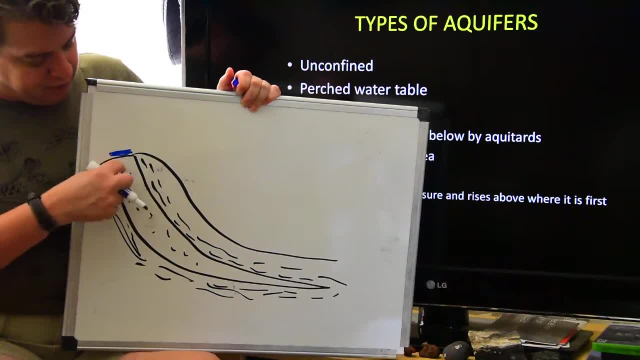 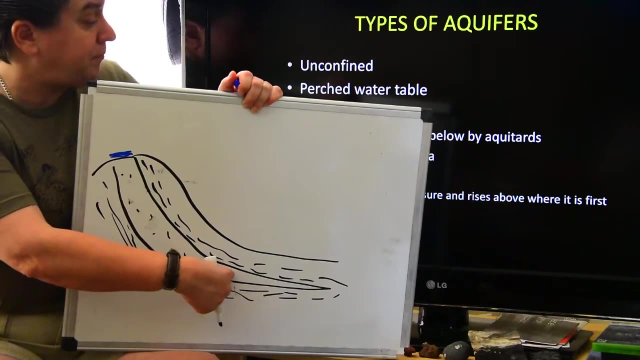 The only place this can be recharged is right up there, Because if it rains out here, that water will infiltrate and then it will hit that impermeable shale and it will never be able to reach our aquifer rock. So the only place where water can enter the aquifer- 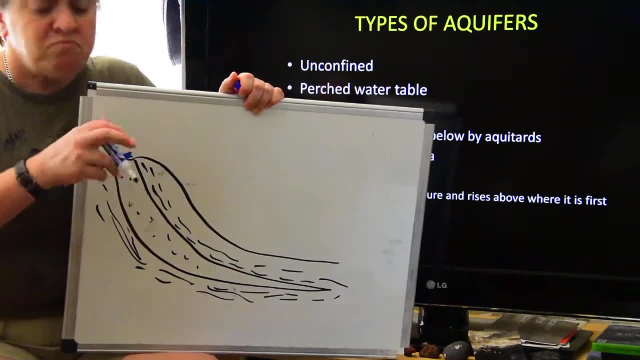 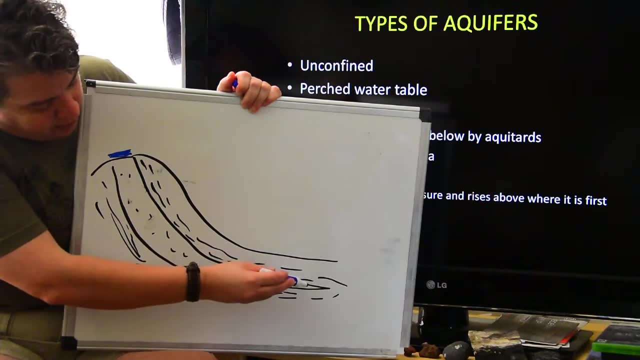 is in this small recharge zone, But, let's say, plenty of water enters there. This water is going to migrate downwards and it's going to reach the end there where it's stuck because it's surrounded by impermeable material. So this water is going to start. 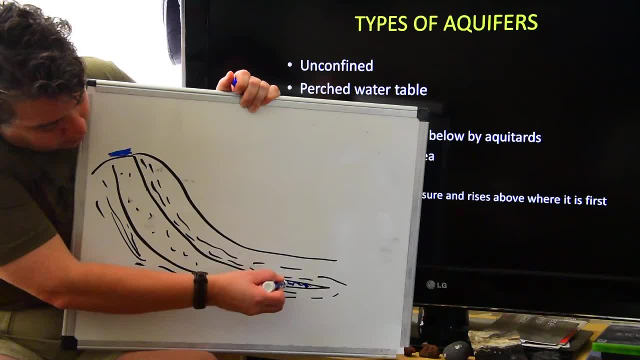 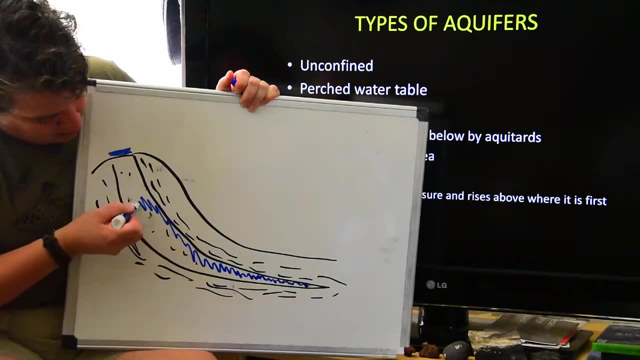 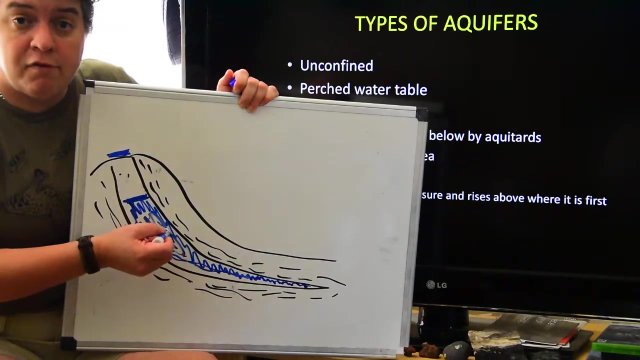 accumulating in this aquifer. We're going to start getting water filling up this aquifer And maybe enough water infiltrates to fill it up all the way to here. So now all of that part of the sandstone is saturated with water. Well, what this can do. 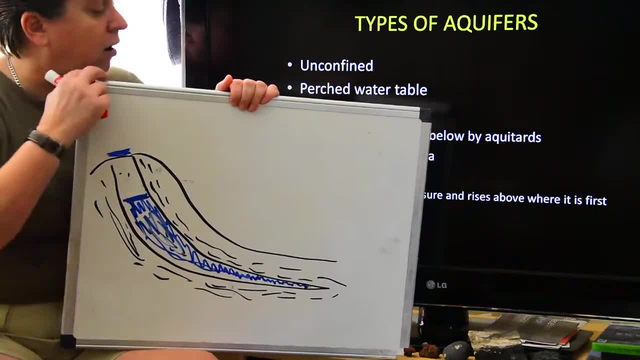 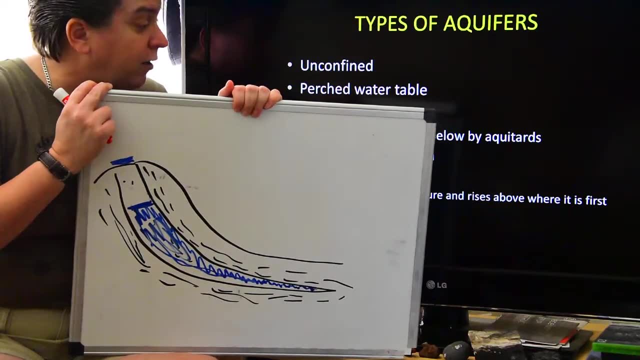 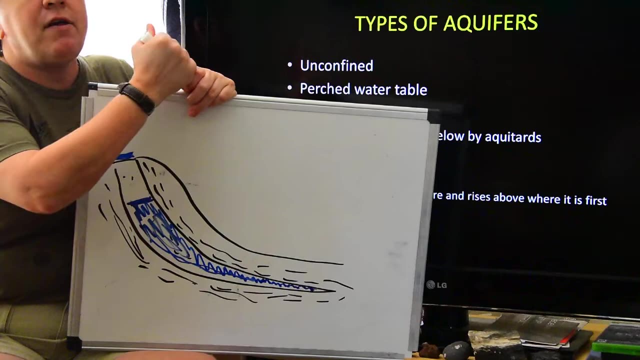 this can lead to what we call an artesian aquifer, And in an artesian aquifer the water is under pressure and it rises above where it's first encountered. So the way this gets under pressure is the water levels all the way up here. 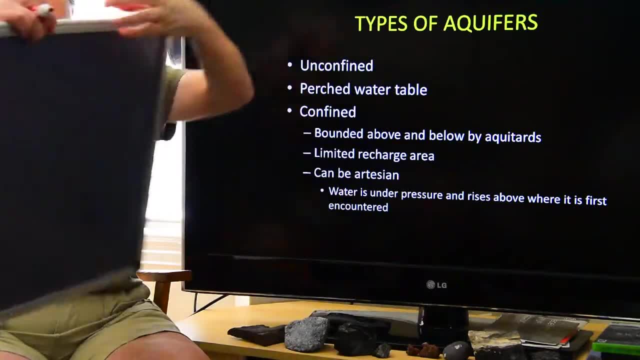 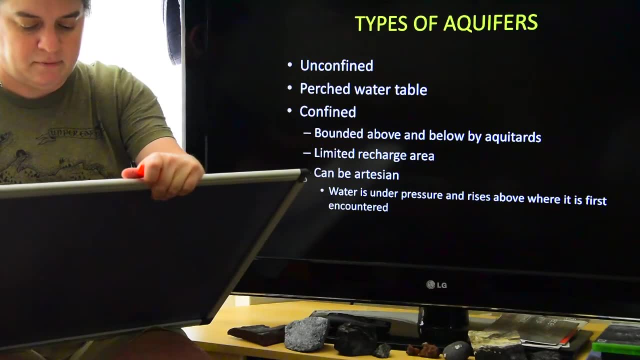 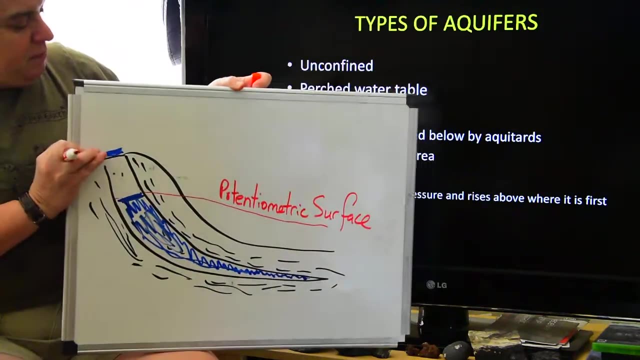 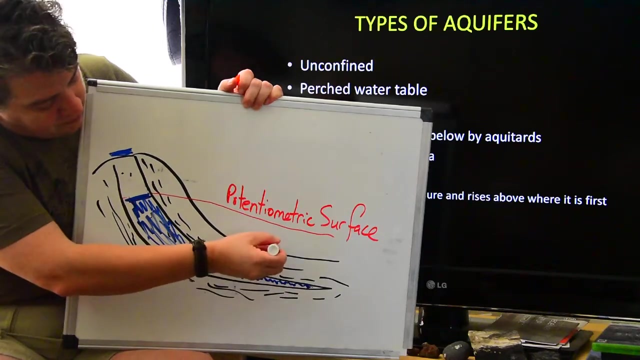 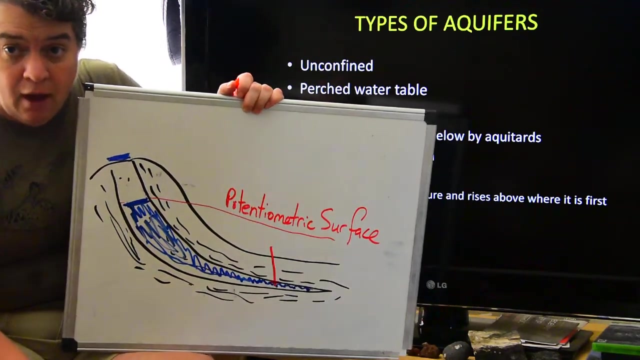 And that sets up something that we call a potential potentiometric surface, And this potentiometric surface is a pressure surface. So what happens then? if you drill a well out here? You run into the water down here, But the water levels all the way up here. 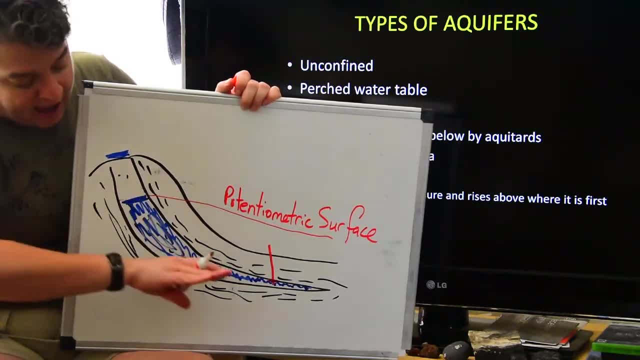 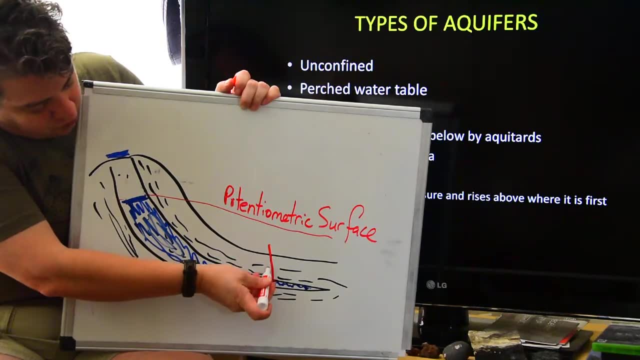 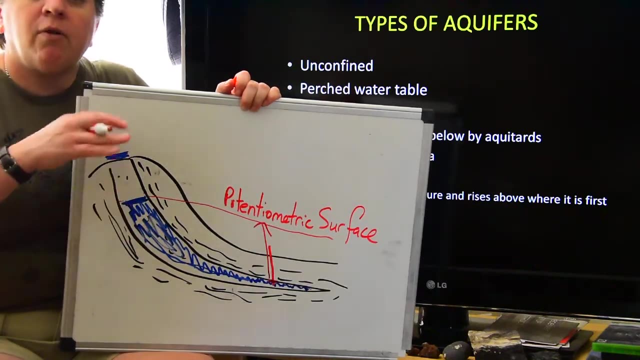 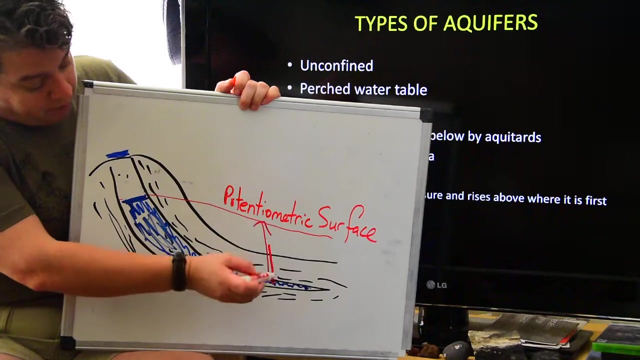 all this water is pushing down on this water where it's encountered, And so that pressure then pushes this water up to the pressure surface. So that's what we mean by artesian: The water is under pressure, and so it rises above where it's first encountered. 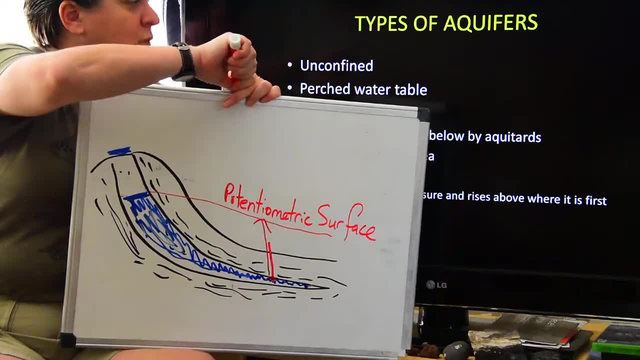 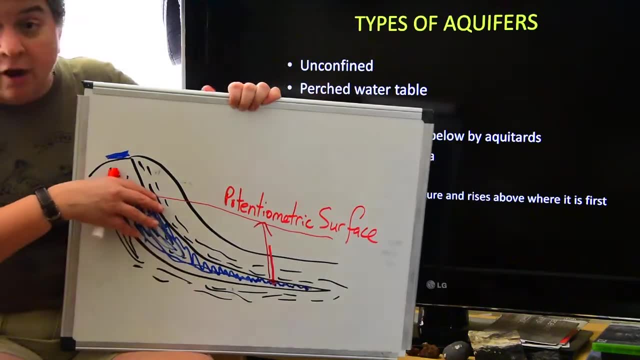 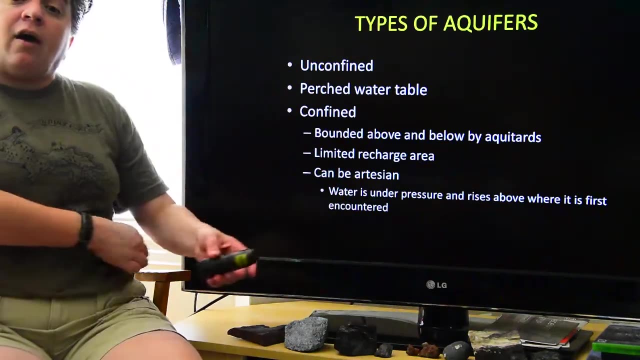 And that can only happen in one of these confined aquifers, because that allows the water to get filled up like this. Alright, so those are some of our basic types of aquifers that we have: The unconfined, the perched water table. 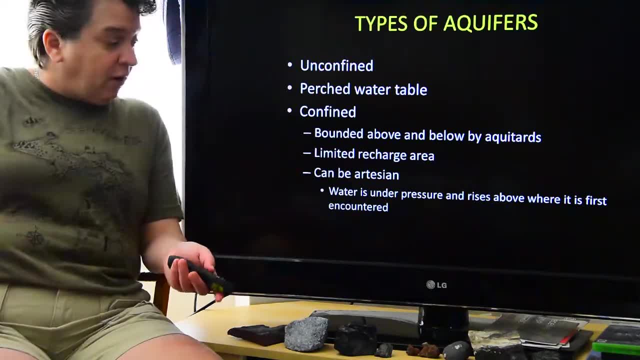 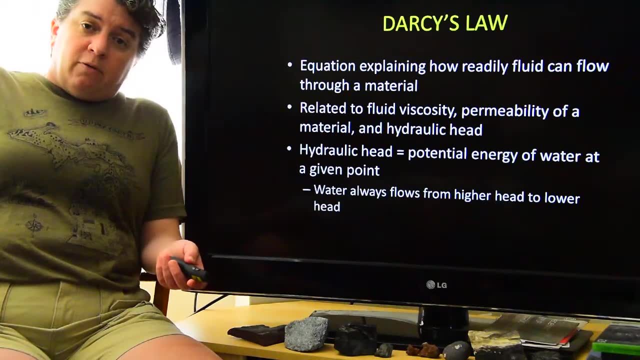 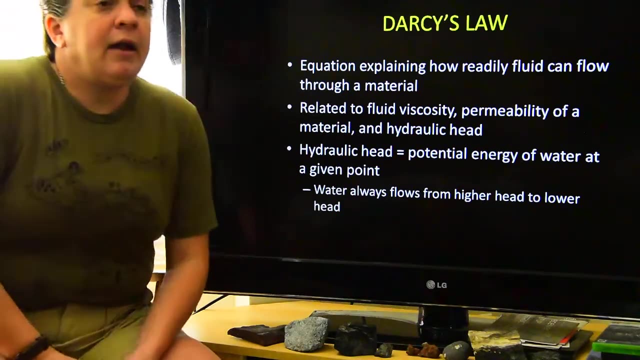 the confined aquifer. that might be artesian And earlier I mentioned that water flows in aquifers. right Water ends up. it's not just sitting down there, it is moving around down there And back in the 1800s. 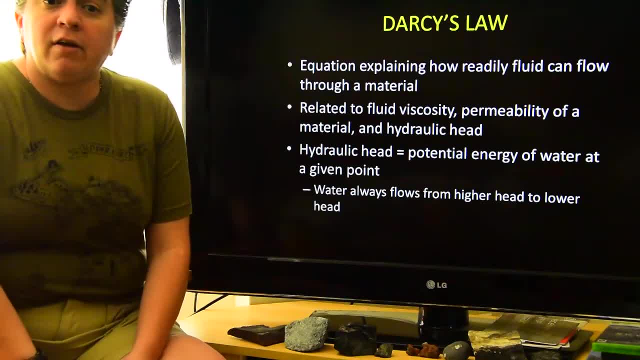 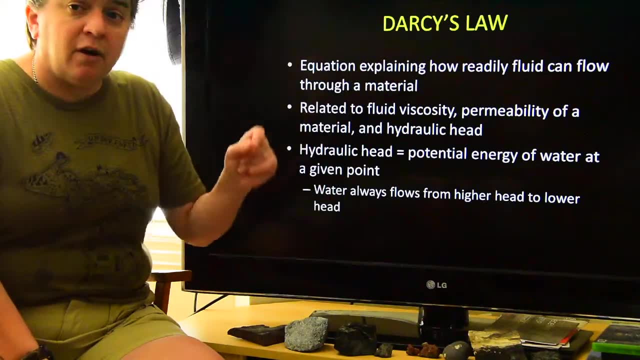 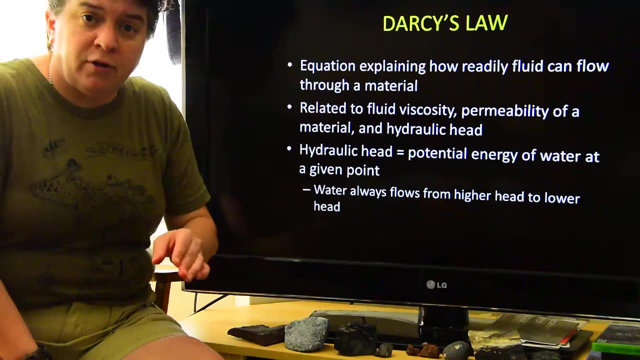 there was a Frenchman who was interested in figuring out how water flowed, And his last name was Darcy. So Darcy developed an equation to explain how readily fluid flows through a material- And we say fluid right, Because this doesn't only apply to water. 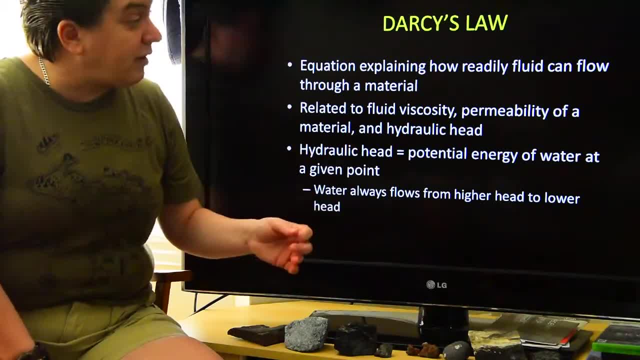 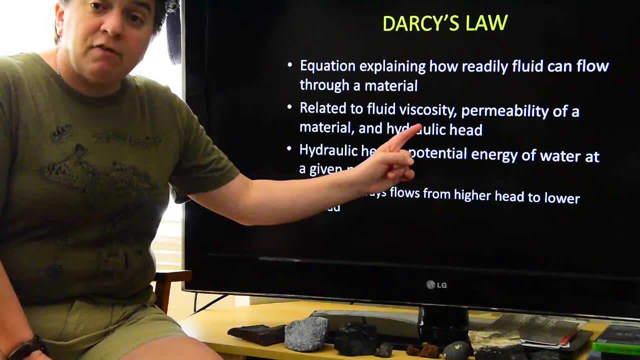 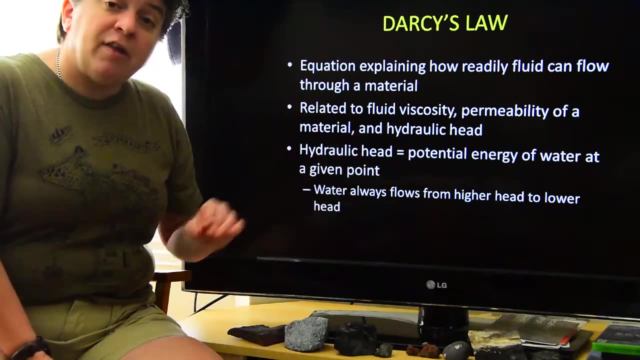 this can apply to things like oil and natural gas as well, So this ends up being related. this equation is related to the viscosity of the fluid, the permeability of the material it's moving through, and something called hydraulic head. Well, hydraulic head. 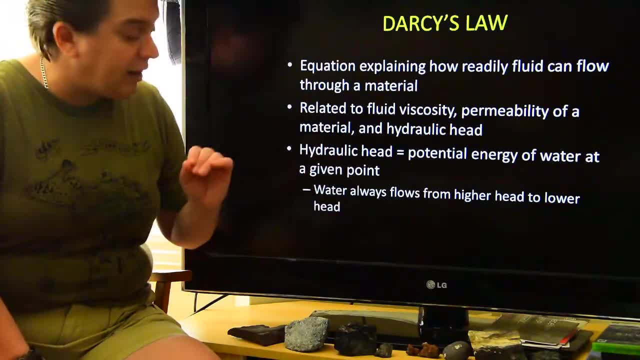 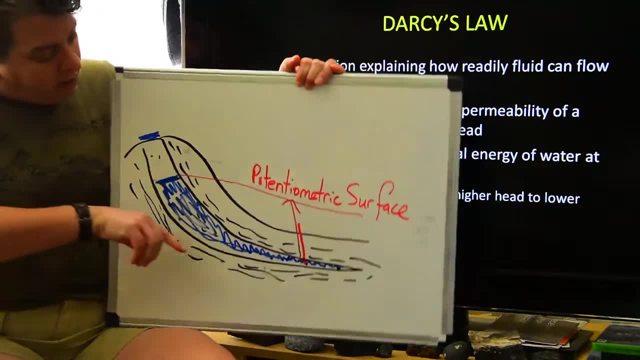 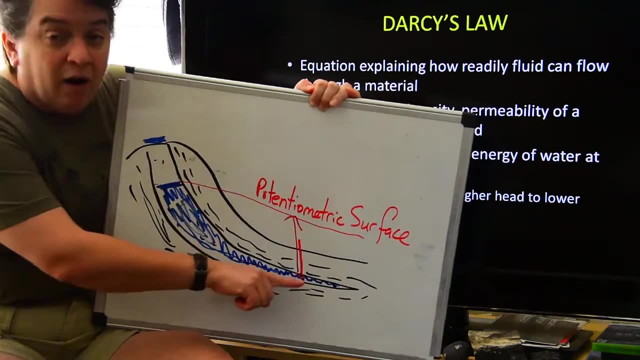 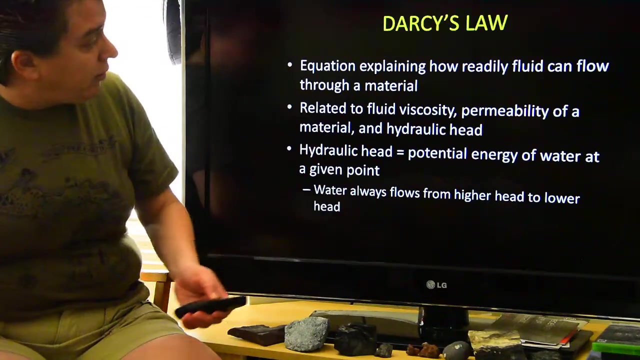 is the potential energy of water at a given point. right, Water always flows from higher head to lower head. So when we encounter the water here, but the water level is actually up here, that's really our hydraulic head, That difference between those water levels. 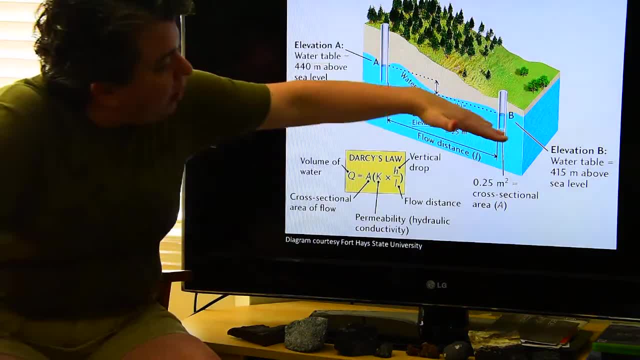 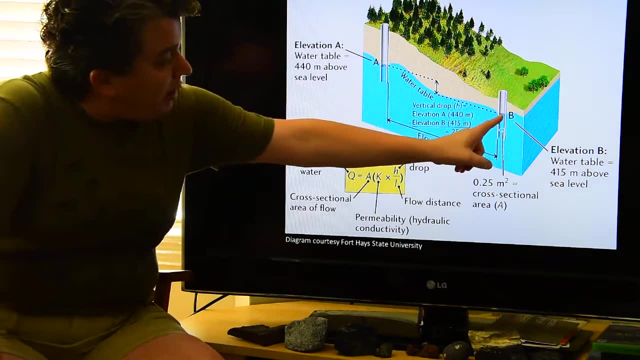 So that's what we're seeing right here. Here's our aquifer, alright, And then we have one well here and one well here. There's our elevation at A, there's the water elevation at B. So the way Darcy's Law works. 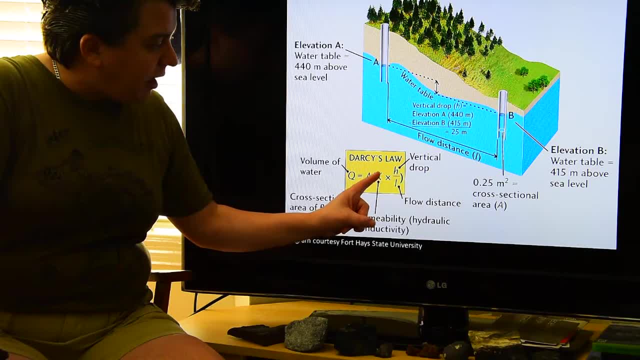 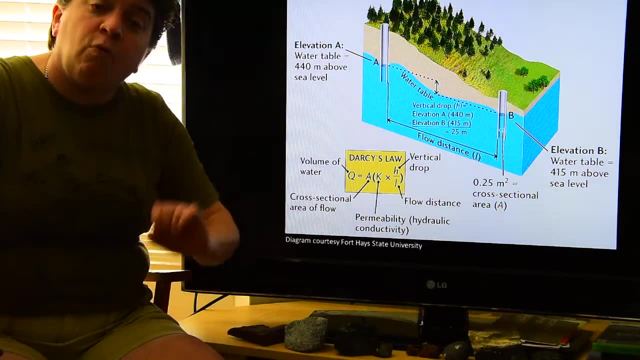 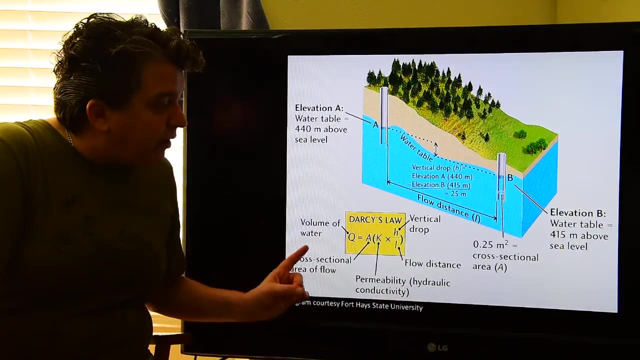 Darcy's Law is: Q equals A times K, times H over L. What do all of those things mean? Q is going to be the volume of water flowing through an area. A is the cross-sectional area of flow. So how big is the area? 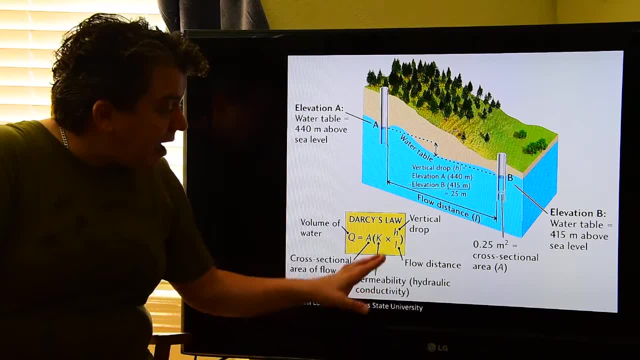 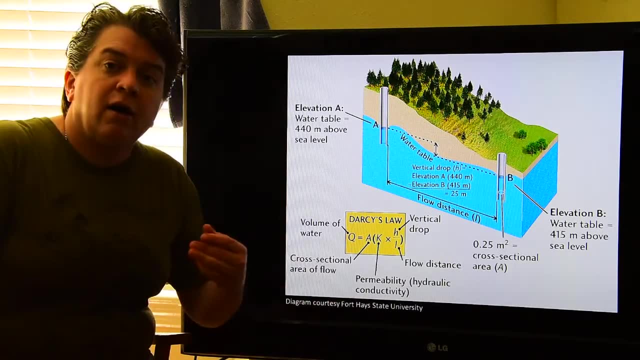 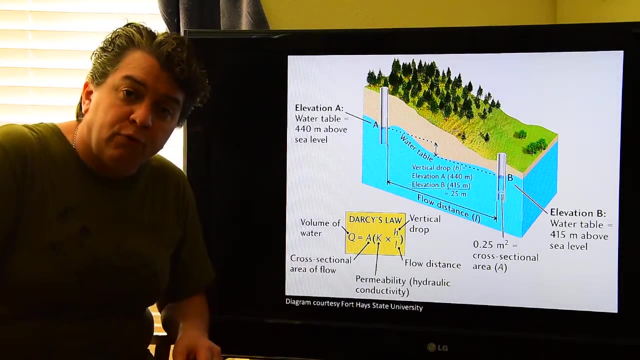 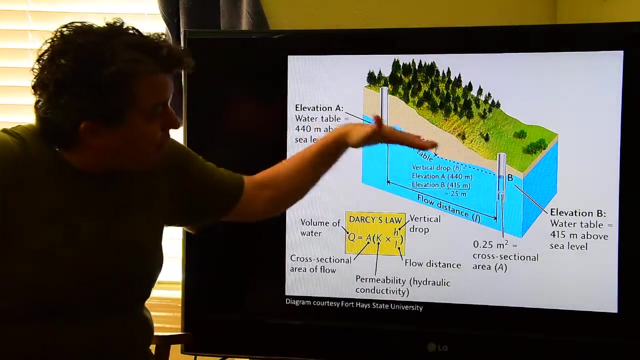 that this water is flowing through. K is permeability, That's hydraulic conductivity, And so this is going to. it relates to how easily those fluids flow through that material. Now H is that hydraulic head right, That's the drop of the water. 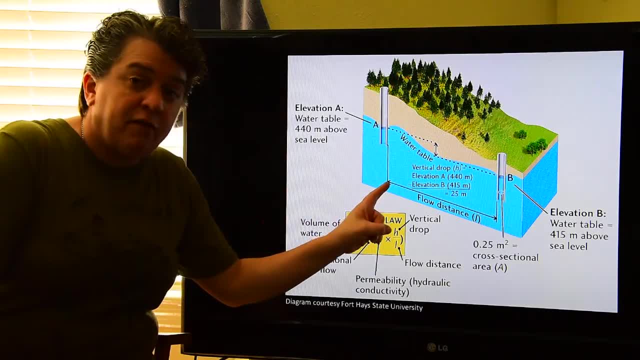 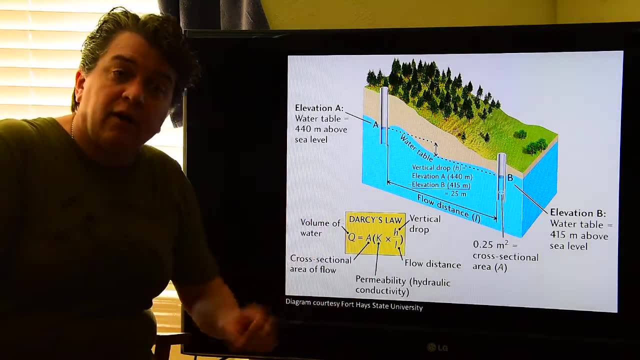 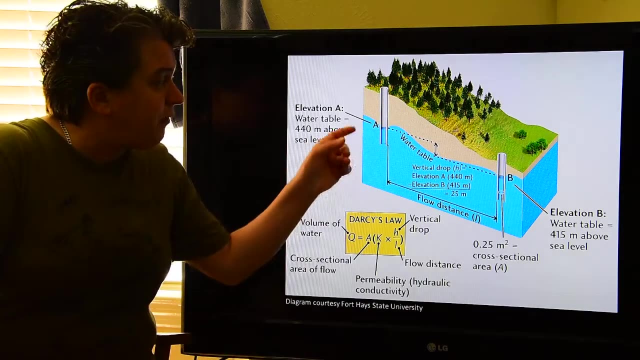 from here to here, And then L is the distance from where we measure one H to the other, And so it ends up, even though it looks like a complex equation, it ends up actually just being simple multiplication. right, You just figure out what the